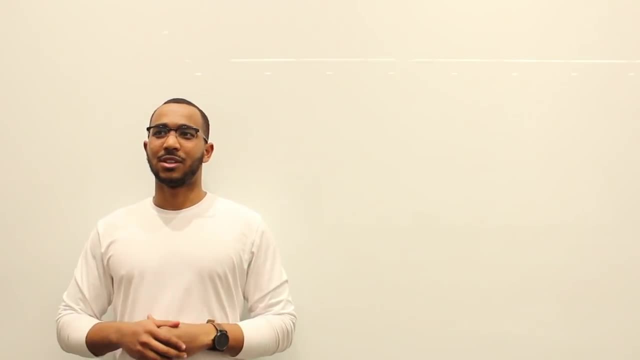 away And I mean it was spring break and stuff And you know. anyway, we are back, sort of refreshed to approach this channel again and continue with the content. And one thing that was kind of surprising is this channel hit 10,000 subs over break, which was kind of cool. 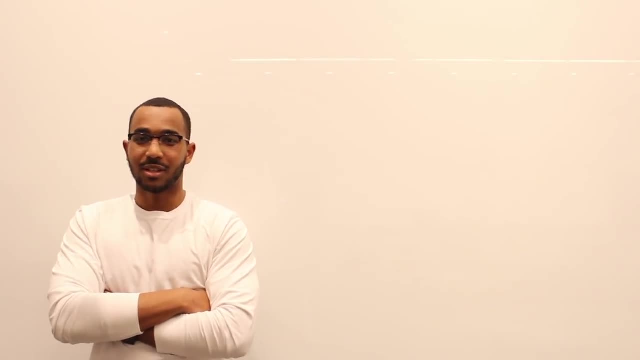 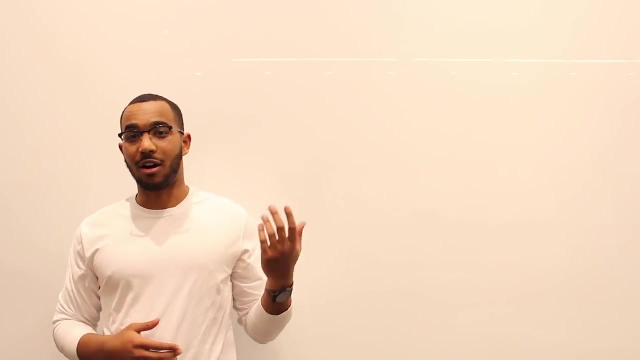 And I didn't even know that would happen. And I came back and I was like, oh, that's kind of cool. And also, a lot of people have been messaging me. Well, not a lot, but a good amount of people have been saying they were getting offers. I'm getting messages from people. 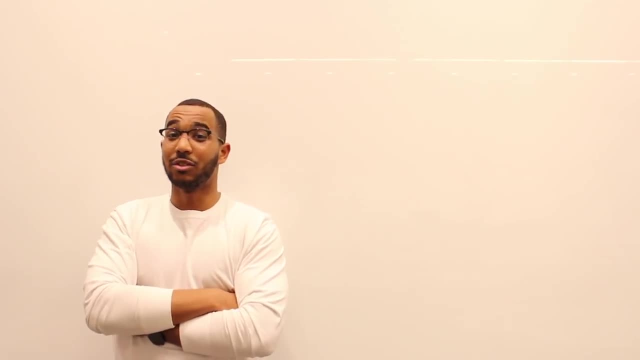 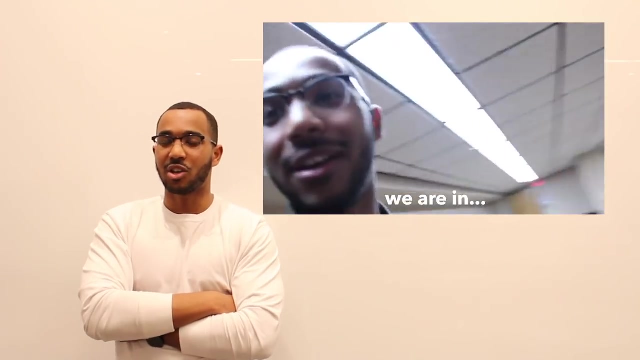 And you got to understand when I started this. I started this literally like doing videos in basements: No one was watching. 10, 20 people were watching And I just kept doing them because I just thought this was necessary. And you know, it's just really cool to actually see it result. 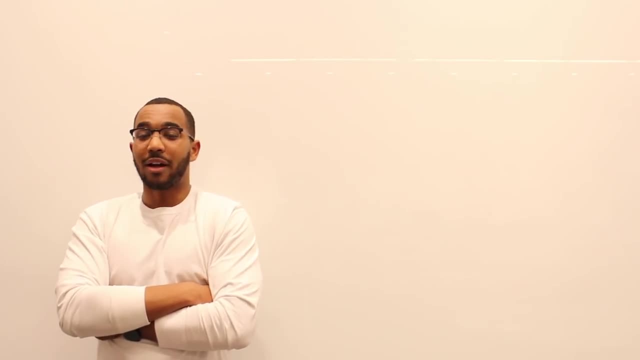 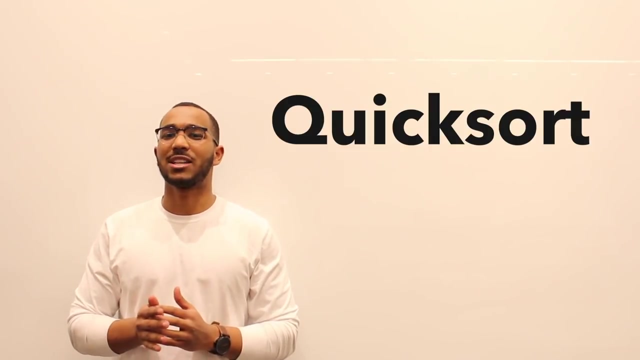 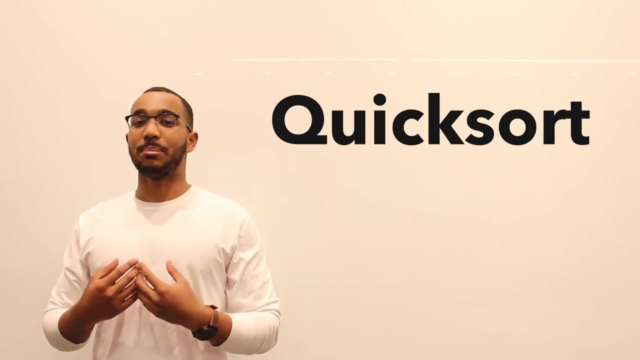 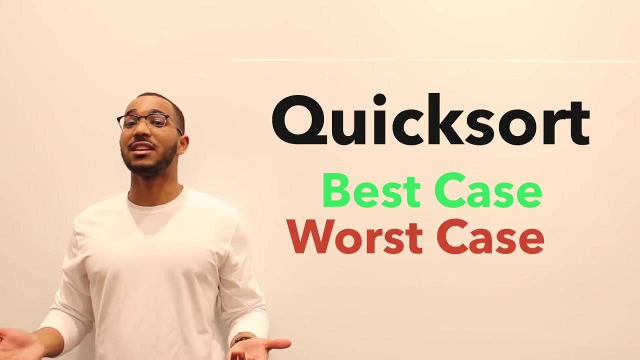 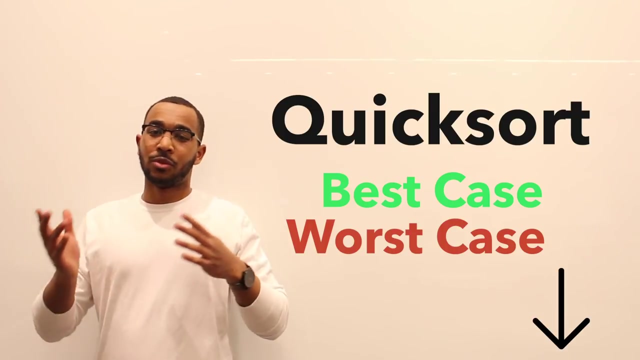 in something. So if this has ever impacted you, please let me know in the comments And I'll see you in the next video. Bye, How does it work? And again, there's code in the description. investigate the code, investigate the explanation. look at both of them So you can deeply understand these things. 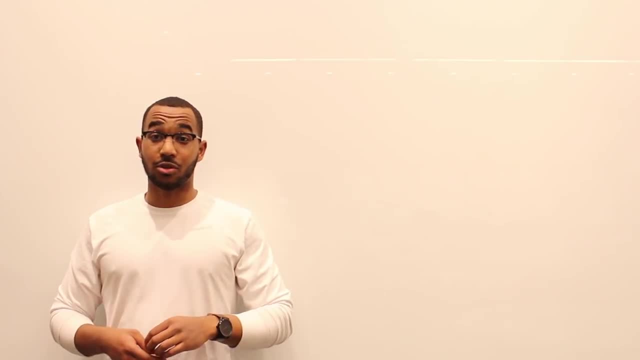 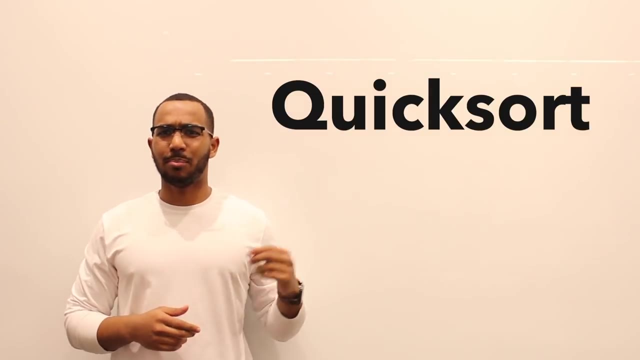 So what we're going to do is we're going to start by introducing quicksort and we're going to do that right now. Okay, So whenever we discuss quicksort, we talk about pivot elements, We talk about partitioning, We talk about- you know how this is recursive or is modeled recursively. 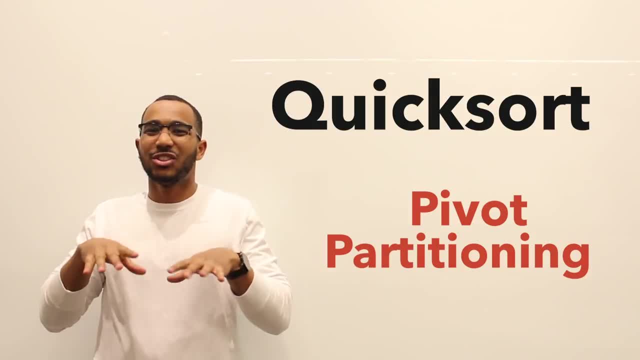 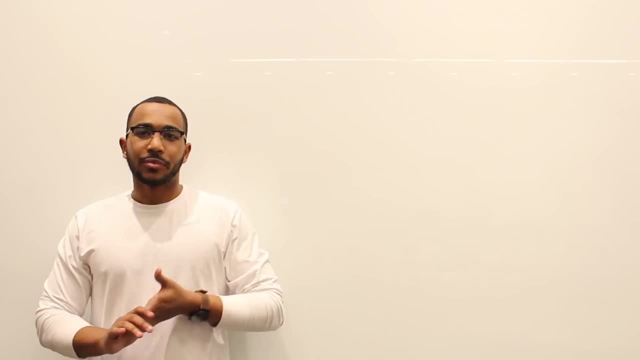 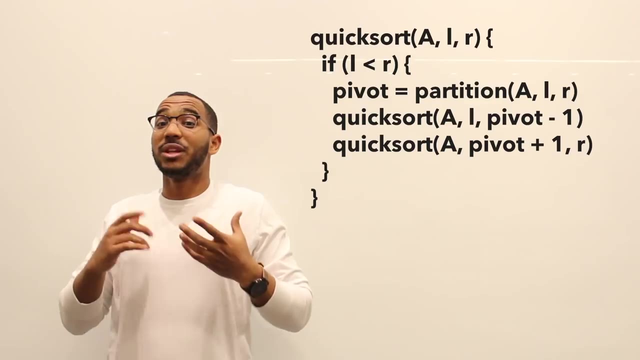 often. So what we need to really dig into is how we're going to be able to do this, And I'm going to- is: what do these things really mean and how does each term relates to the algorithm as a whole, So quicksort. quicksort has two major subroutines, or routines of sorts. It has the split function. 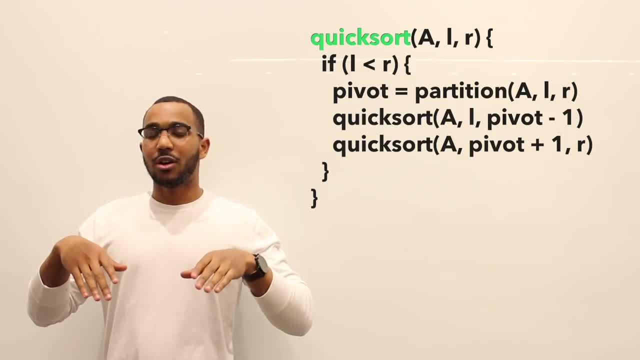 or the quicksort function that splits the input, calls the partition step first And then, based on the pivot, we get back from the partition step. We split the data and run our trees going left and right, And you'll see what I mean. We don't need to do that. We don't need to do that, We don't need. 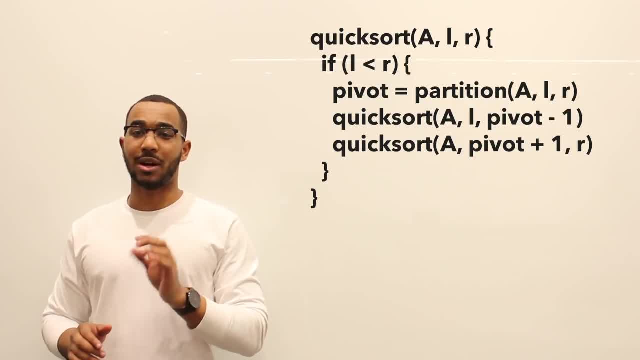 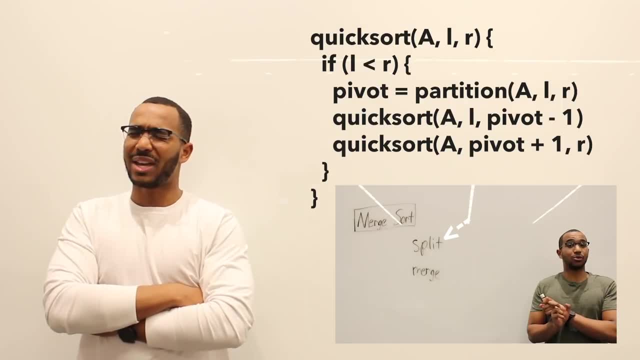 to know what a pivot is. We don't need to know any of this, Just follow with me what I'm saying right now. So that's the quicksort subroutine. That's the splitting routine. Remember, back to merge sort. we had a merge subroutine and a split subroutine. So we're discussing the split. 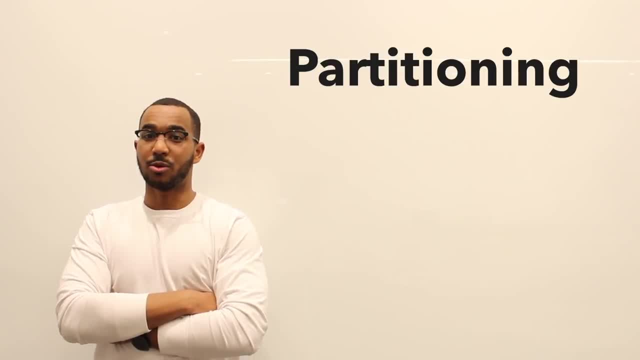 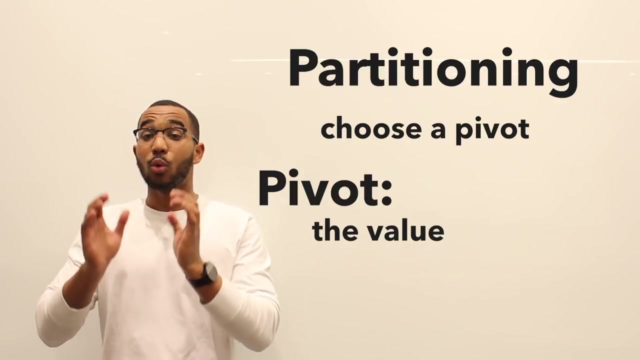 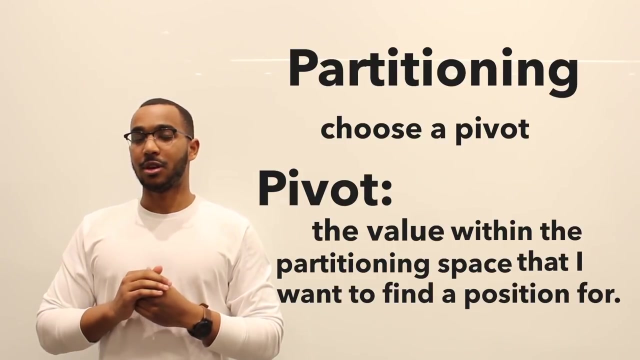 subroutine right now, And then we have the partitioning subroutine. So the job of the partitioning subroutine is to choose something called a pivot. So what a pivot value is? it is the value within the partitioning space that I want to find a position for. So what we need, 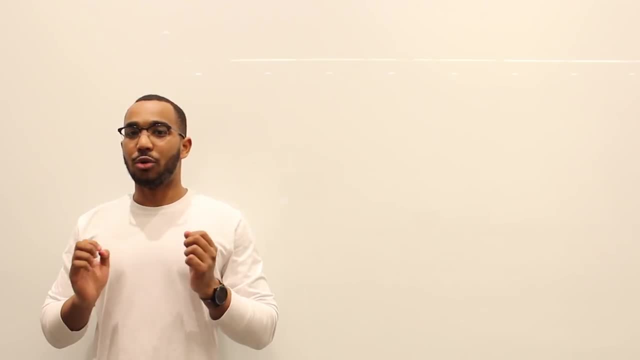 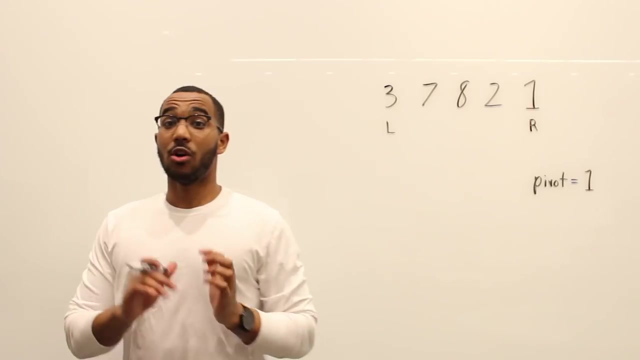 to see is we need to see a concrete example. So let's go through a partitioning example so that you really can see how this works And you don't need to understand any of this right now. I'm giving you high level overview. We'll go in depth later, So let's look at that right now, Okay, So, 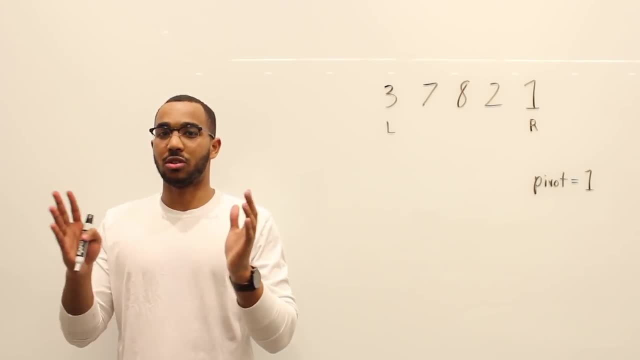 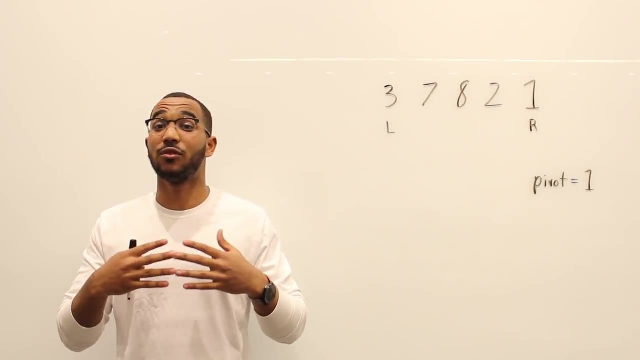 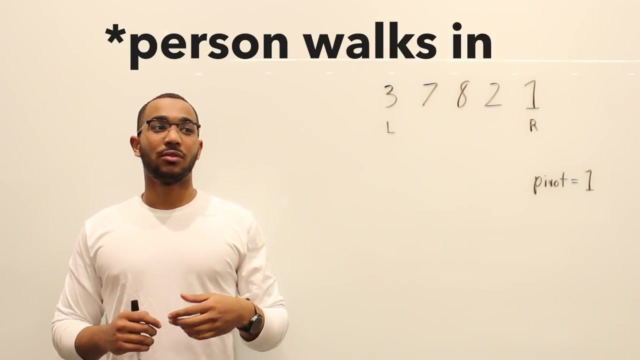 what I said. the space that we're going to partition against the space that we're going to be looking within so that we can move items to find a position, for the pivot item is going to be have a left bound and a right bound. So, oh, it's fine. So imagine this When we start our space: 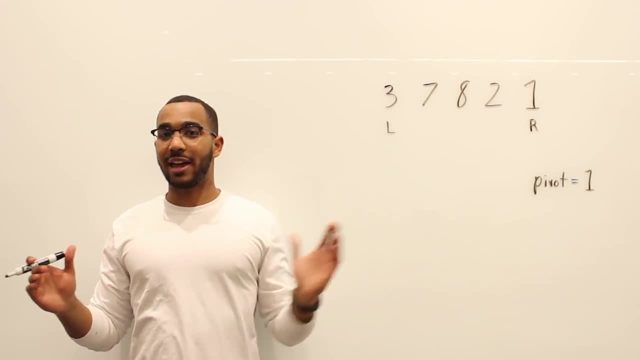 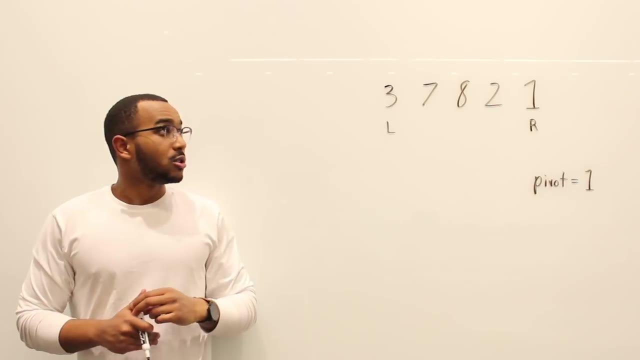 that we partition against is going to be the whole array. The left is at zero, The right is at zero, The left is at zero, The right is at zero, The left is at zero, The left is at zero, The right is at length minus one if we're indexing off zero right. So what we need to think is what? 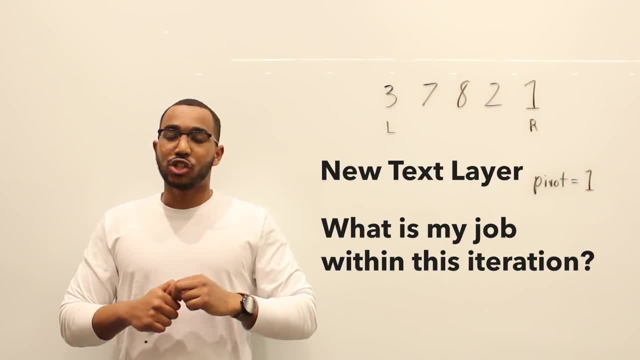 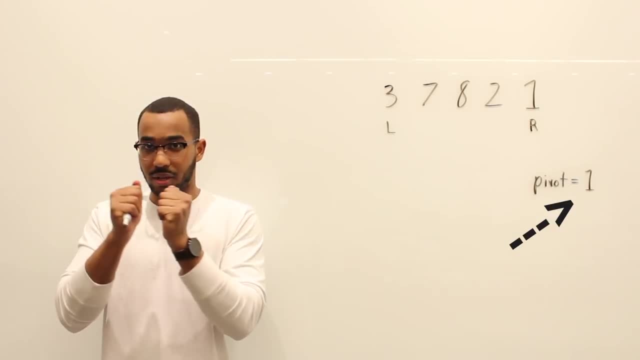 is my job within this iteration And my job is to find the position for the pivot- That is Quicksort's job- within the partitioning subroutine. And when we find a position for the pivot, we return that index of the position so that my split subroutine knows where to chop the array. 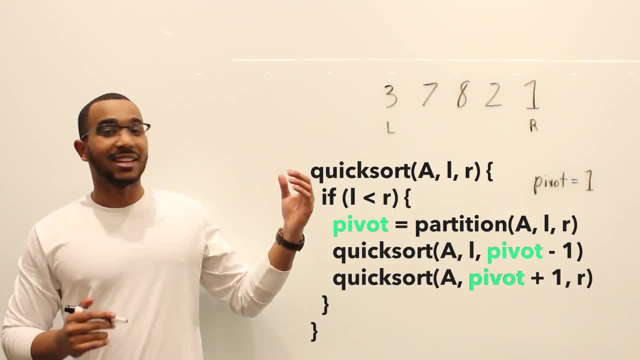 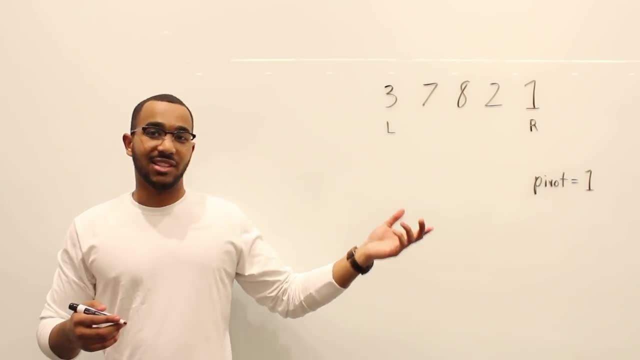 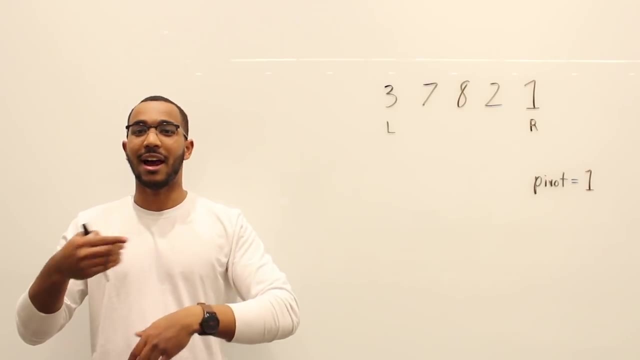 So continue following with me. What we did was we randomly chose a pivot, Some algorithms, you can choose it as the last element. You can choose it as any element. We'll see which is the best element to choose as the pivot when we analyze recurrences and look at the tree and how. 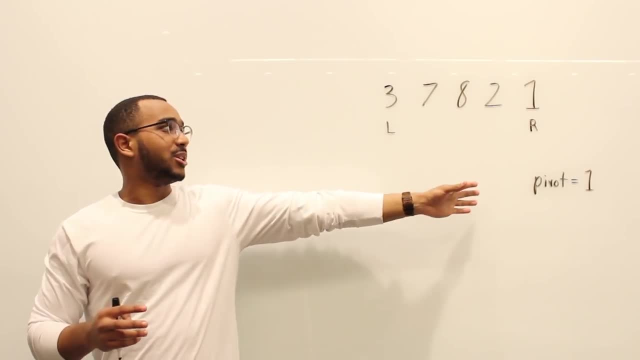 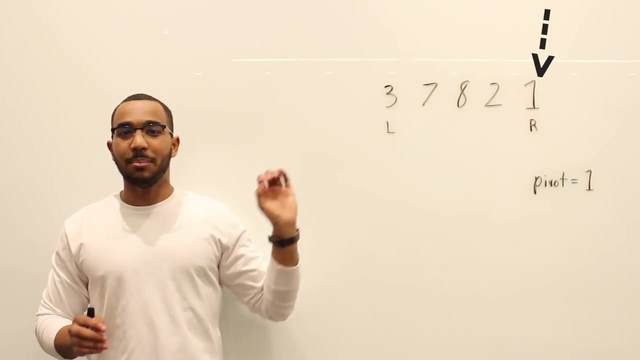 this splits our data, But we randomly said, okay, I want to find the position. one belongs in The position. the last item: When you say pivot, ignore pivot. Pivot's a confusing term. I don't know what pivot really means. Just think of pivot as the item I. 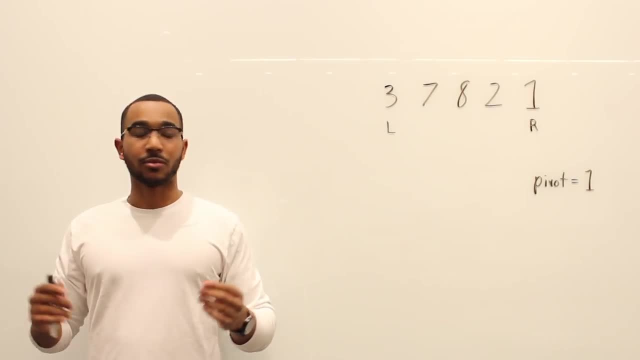 want to find a position for. That is all a pivot is. So what we're going to do is we're going to search the array and we're going to bring all the elements less than the pivot over here, all the elements greater than the pivot over here, and where my pointer at the last placed position of 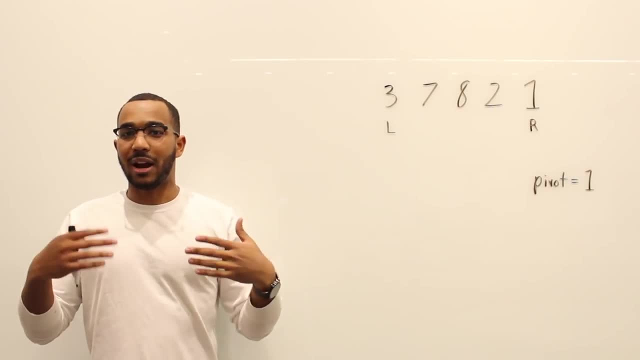 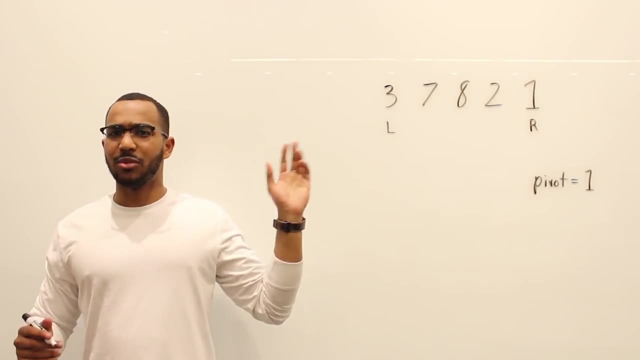 items less than the pivot is going to be. So what we're going to do is we're going to search the. That's going to be where we place the pivot item, And you'll see what I mean. That's confusing in words. Let's just watch an example. So I'm going to let me move the left and right above. I'm 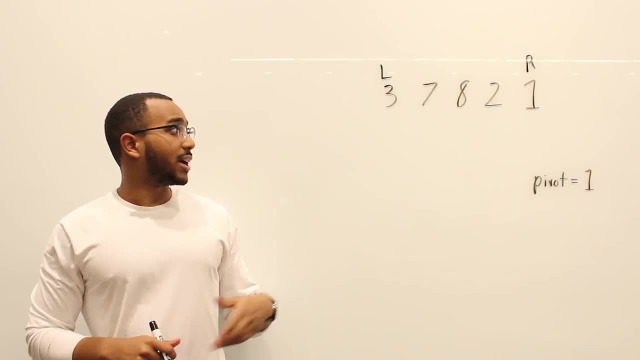 going to have a pointer I. I'm going to set it right here. And I'm going to have a pointer J. I'm going to set it at the same position as I And if you're watching this and you're in my algorithms class, we would index off of one and I would be over here. But just ignore that, Just. 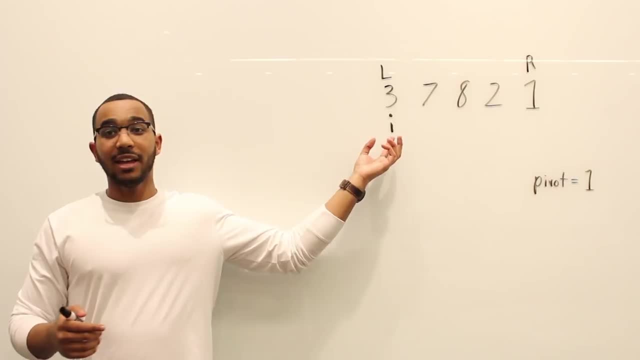 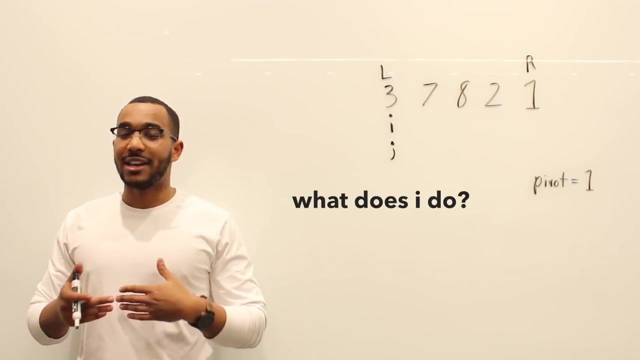 follow the concepts, Ignore the indexing. So I is right there. J will sit at the beginning as well. J is going to start at the left boundary. Where's the left boundary Right there? So what are the jobs of I and J? I's job is to remember. 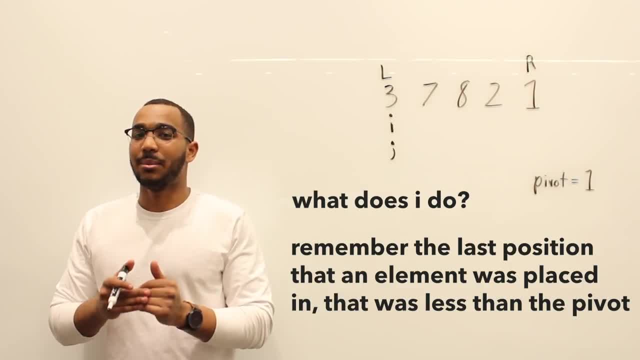 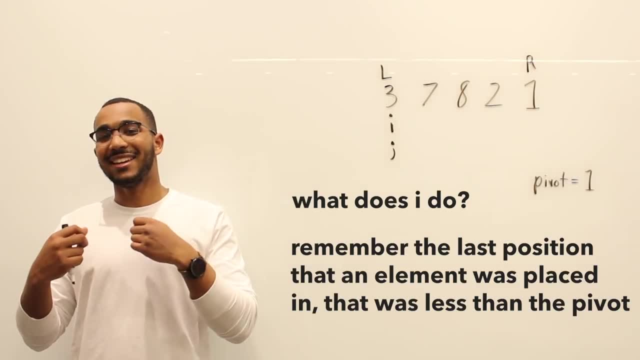 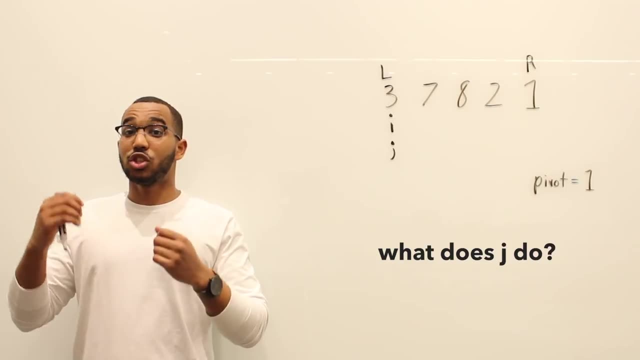 the last position that an element was placed in that was less than the pivot. Again, I's job is to remember what is the index, that I last placed an item less than the pivot. So I'm going to set an item less than the pivot And J's job is. J's job is to scan from the left boundary to the item. 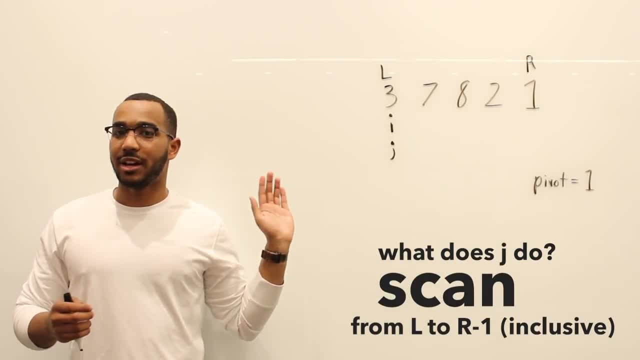 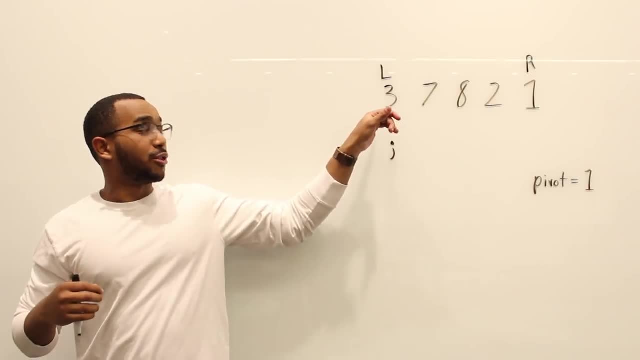 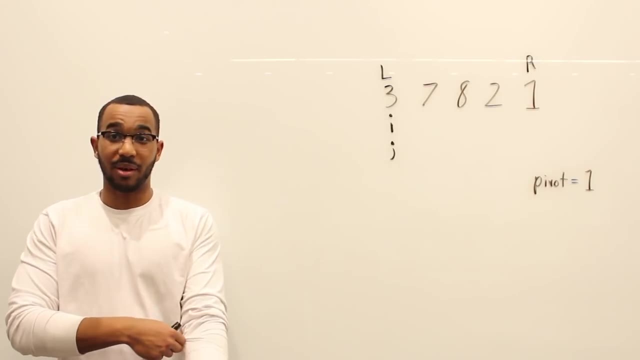 before the right boundary, scan all the items so we can check all of them and see if they're greater than or less than the pivot. So watch this. This is what happens. Three, Remember J, is our searching pointer. Is three less than or equal to the pivot, or is three greater than the pivot? Three is 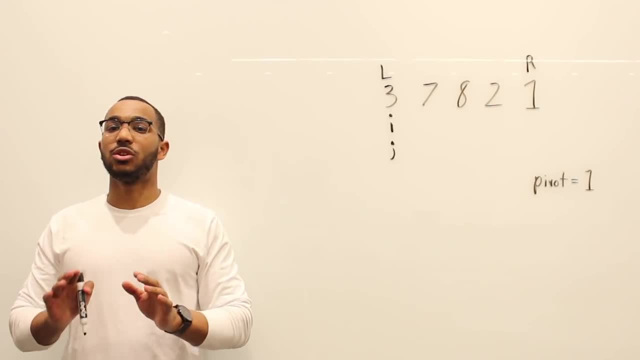 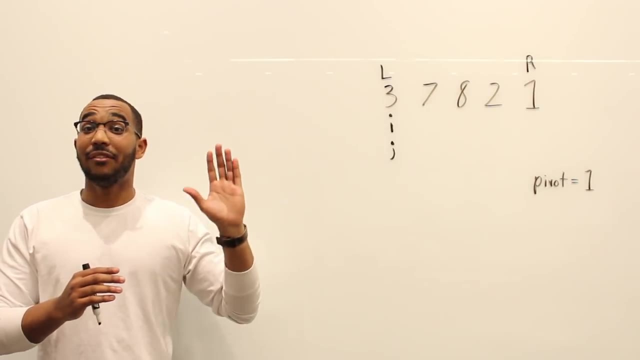 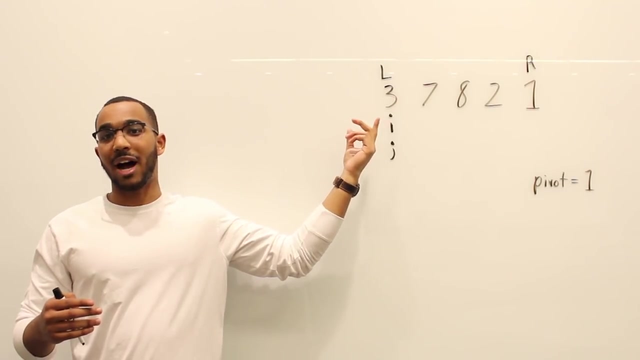 greater than the pivot. So we do not execute a swap. We do not place an item into the section that is less than the pivot. Every item from I and behind is less than the pivot, Or, in this case, every item from I minus one. 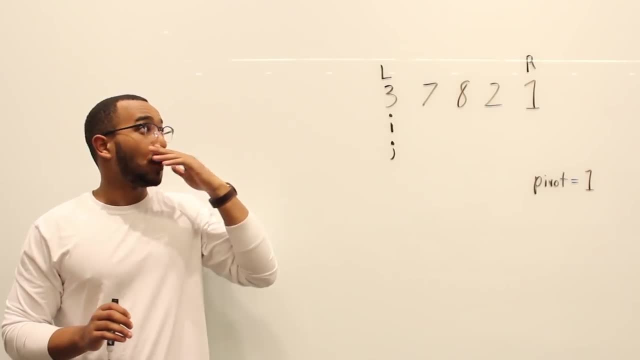 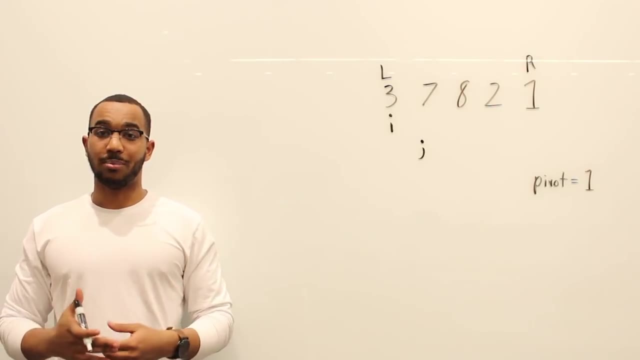 and behind Again, ignore the indexing, Follow the concepts. So three: Three is more than the pivot, So move on. So now is seven less than or equal to the pivot, It's not. So move on. Is eight less than or equal to the pivot of one? It's not. Move on. And now is two less than or equal. 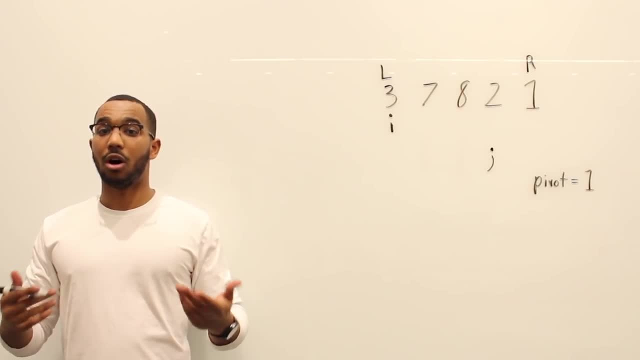 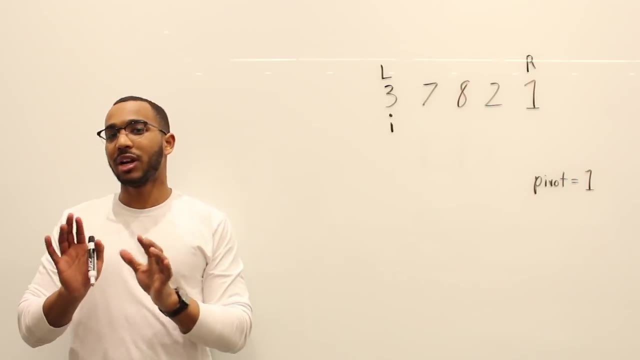 to the pivot. No, it's not, Move on. And we see J is going to hit up against the right boundary, So we finish. We don't do that. And again, if you're worried about the indexing here and how I'm being all loose about it, the code's in the description- Very, I mean, it's code, So you can't. 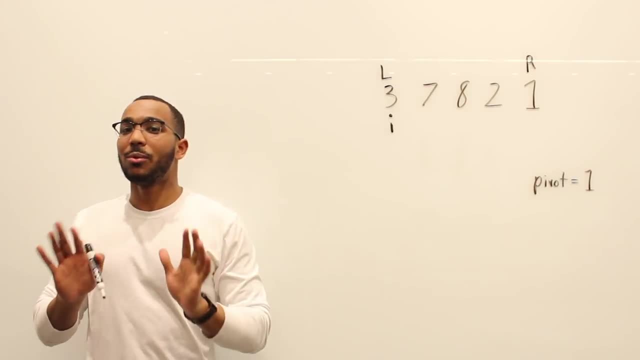 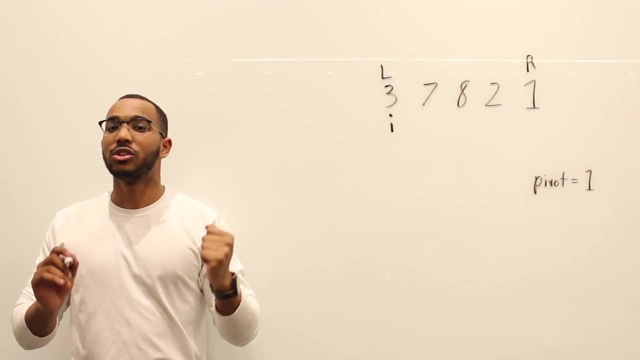 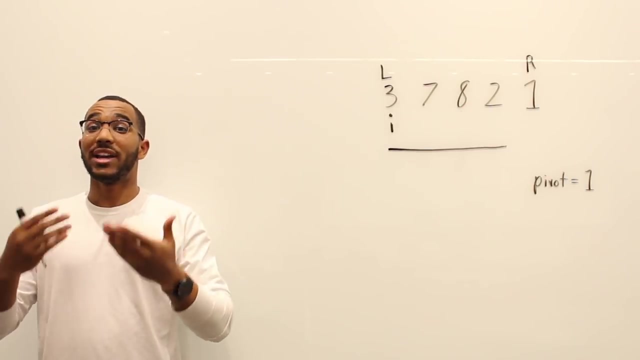 mess around with the indexing. It has to be right. But do you see what we just did? I searched the. every item from the left boundary to right minus one, compared it against the pivot. And what do you see? Every single item here over here that is greater than the pivot. Every single item from. 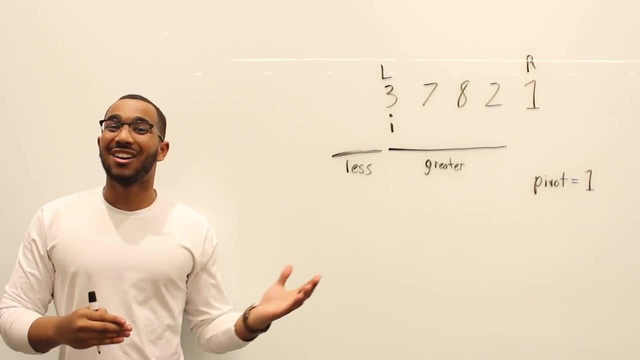 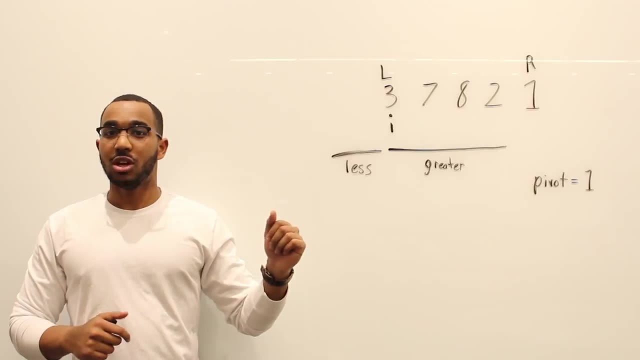 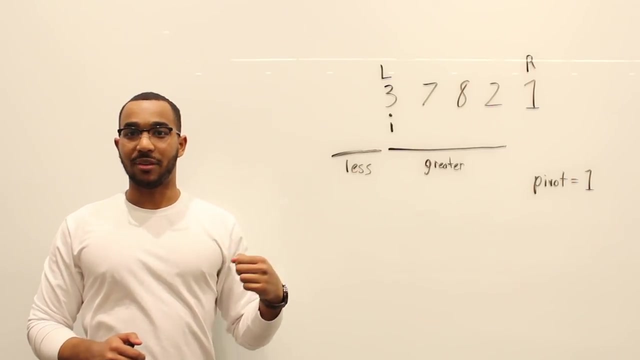 I minus one, and behind those items are less than the pivot. So do you see now why do we swap the item at the pivot position into I? It's because if all these guys are going to be left behind are less than the pivot, all these guys are greater than the pivot. Is this greater than one? Yes, 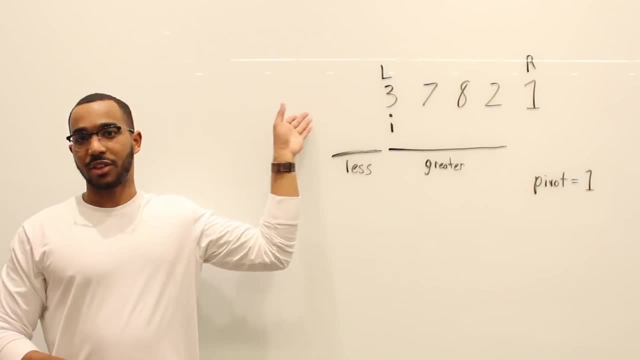 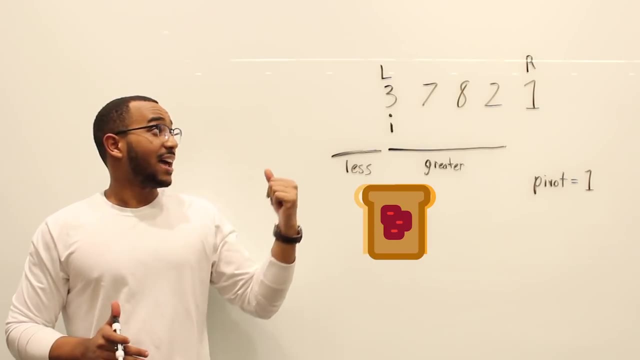 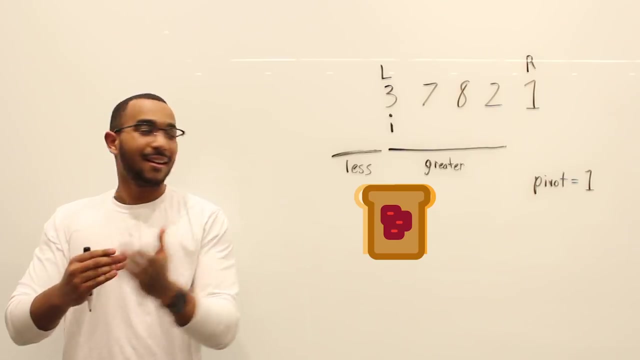 yes, yes, yes, Is this less than one? Well, there's nothing here. What we do is we sandwich it. We sandwich it between the less section and the greater section, And what do we do? We swap between the pivot item and I. I is the ending of the section of items less than the pivot. 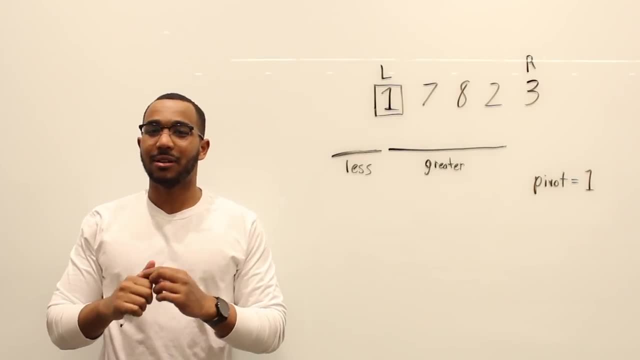 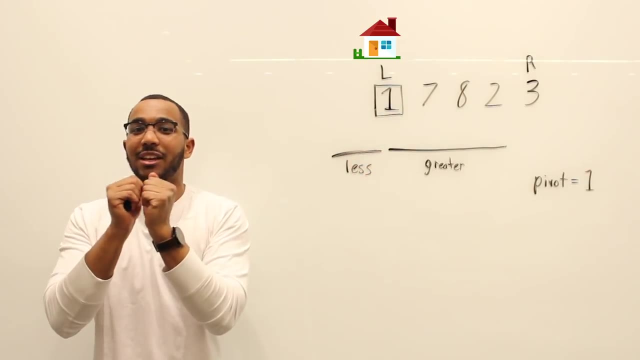 So what happens is this: Do you see what just happened? Our job was find me a home for one. We found one's home by finding- I don't want to say sandwich again, but I mean that's kind of an intuitive way of seeing this. All these items are less. 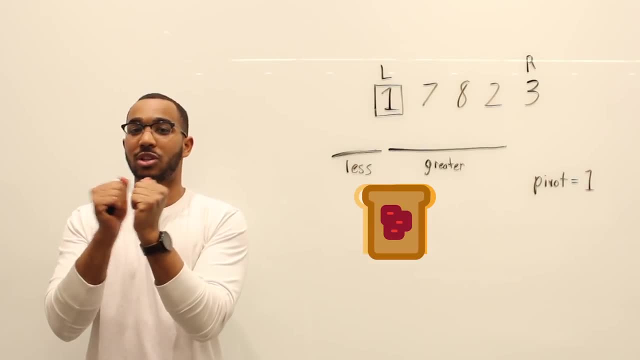 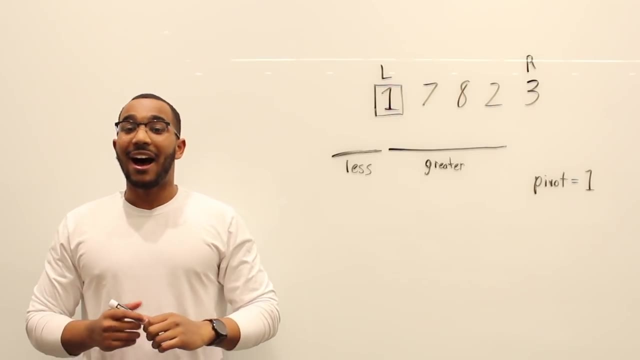 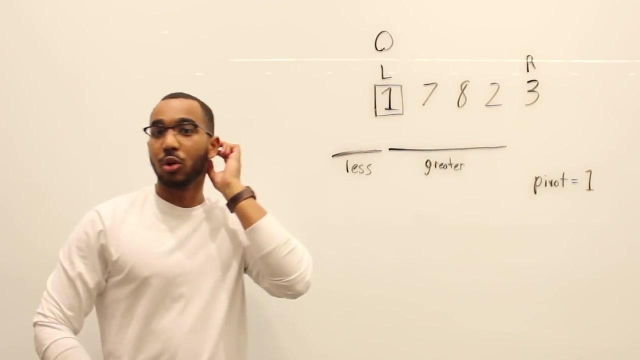 All these items are greater. I sandwich one between those items And now that gives me one's final position. What do I return to my caller? I say, hey, I found a final resting place for the pivot item. It sits at index zero. So what I say is: I found a final resting place for the pivot item. 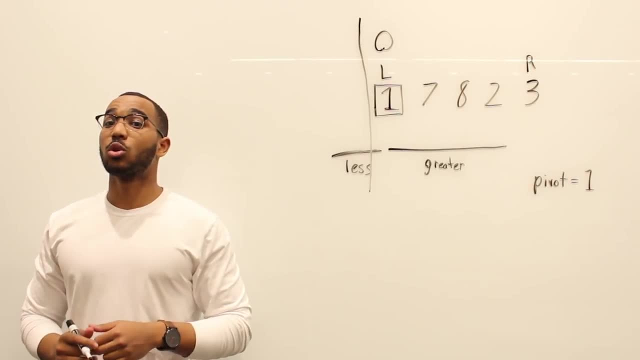 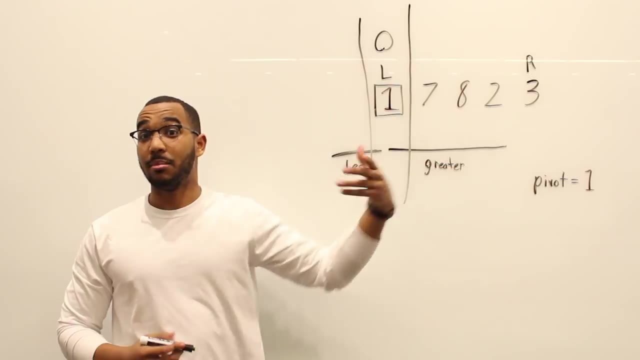 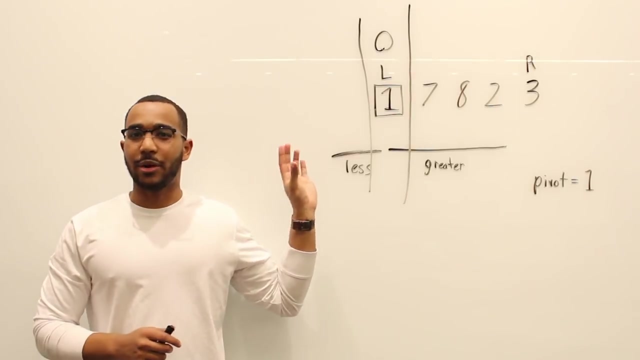 So what I say is run quicksort on the left half, run quicksort on the right half And, as you can see, is this guy is going to base case out And this guy is going to be four items and minus one items. So this is actually special. I did this on purpose. This is special because this is a worst. 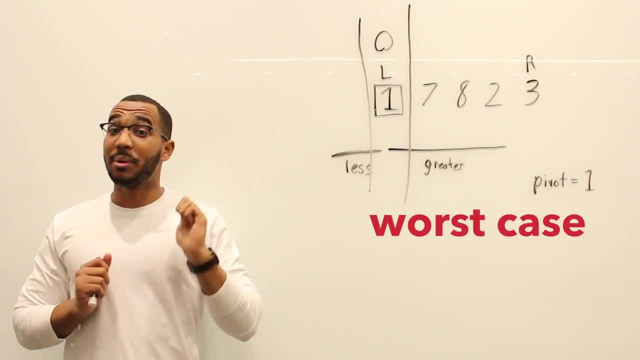 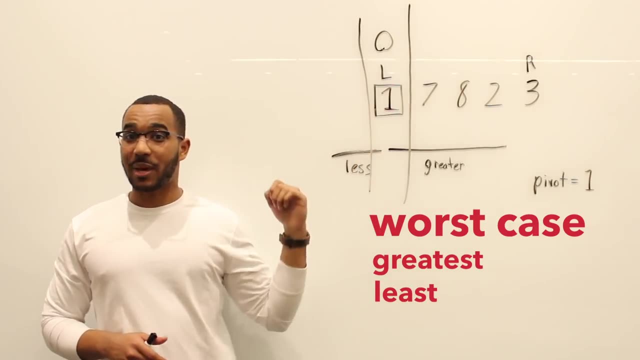 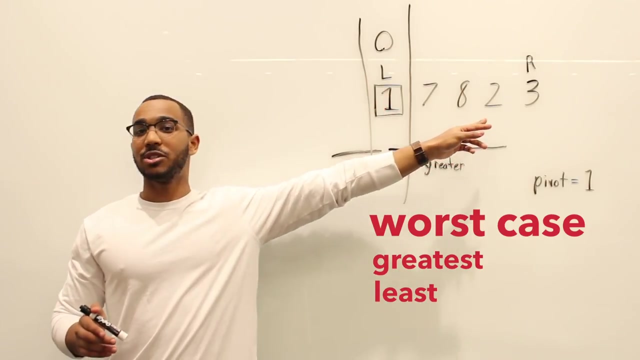 case. This is something I want you to take note of. If the pivot is the greatest item or it is the least item, what happens In my partition space? the least item is going to be all the way over here, Or if it's the greatest item, I'll find a. 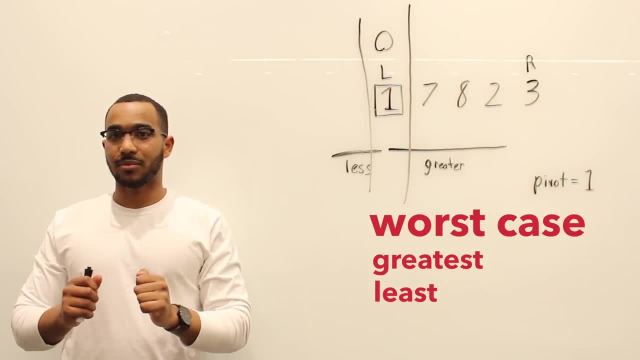 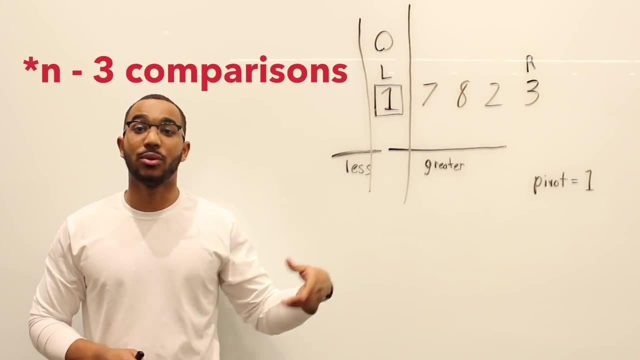 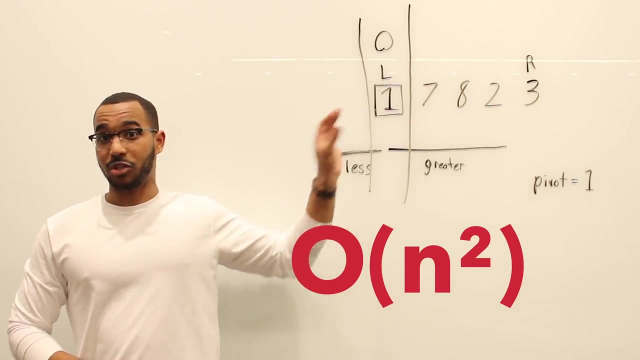 position for it on the right boundary. But the problem is I unevenly just chop the space, So I'm going to do n work here. Next call we'll do n minus one, n minus two, n minus three. And this is why the worst case of quicksort is n squared. When you pick bad pivots, this is a bad pivot. we. 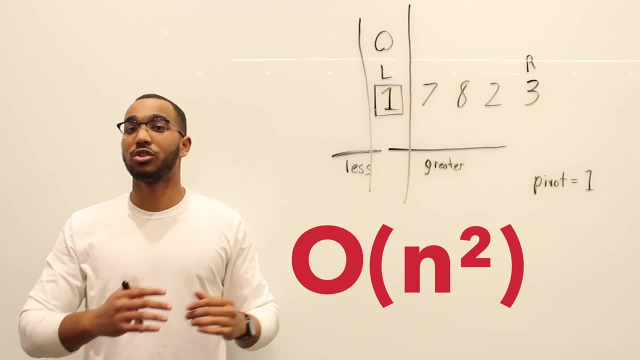 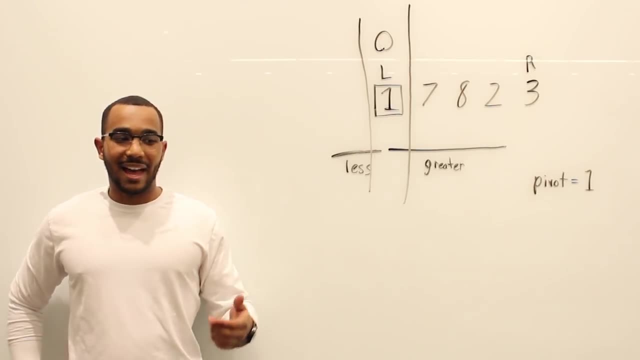 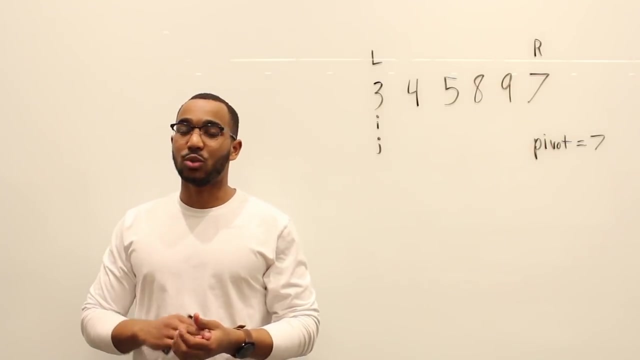 just chose. We're going to be approaching doing quadratic work And we'll analyze the tree Like any of this, But now that we saw that, let's look at a better example of what quicksort is going to do in a nicer case. So what I just showed you was a worst case. We chose a very bad pivot And then 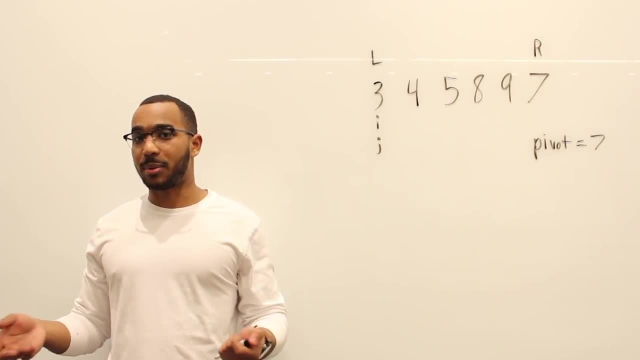 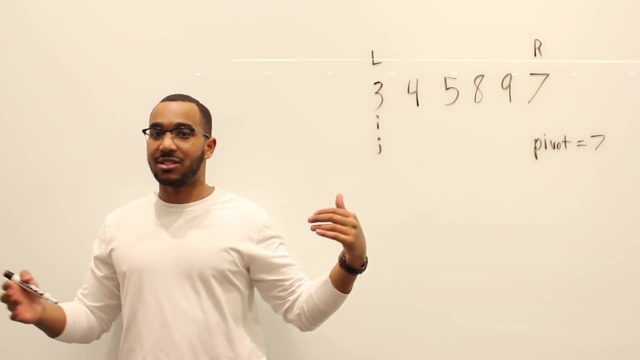 I'm going to have a potential of doing n squared work because I'm not splitting this evenly, And again we'll see that later. So here's a nicer example. We pick the pivot as the value of seven. Again, you see me picking the last item. You don't have to pick the last item, A very pivotal thing. 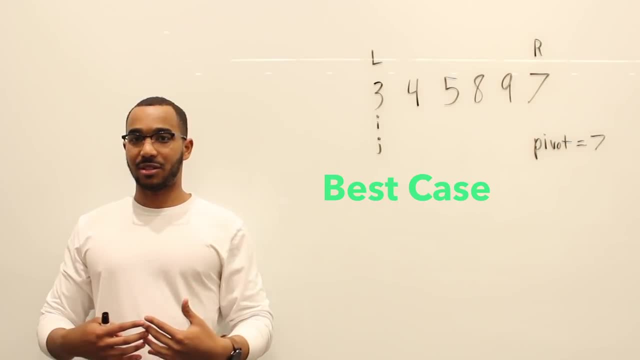 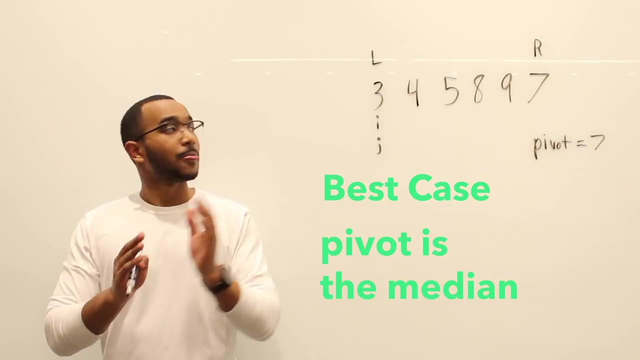 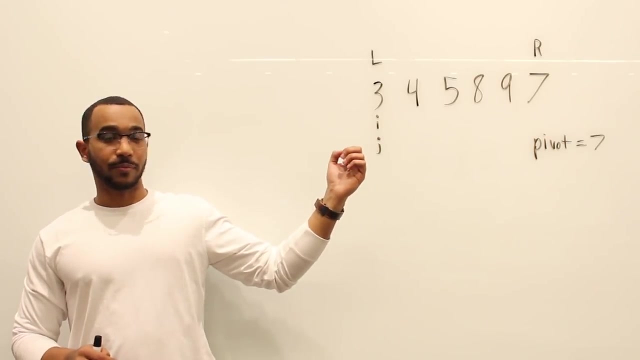 if not unintended, is that we pick a good pivot. The best pivot is when the item is the median of the partition space. So our partitioning space, or the space that we're going to look at, is going to be the whole array left and right boundary. Again, I start J on the left boundary And I can: 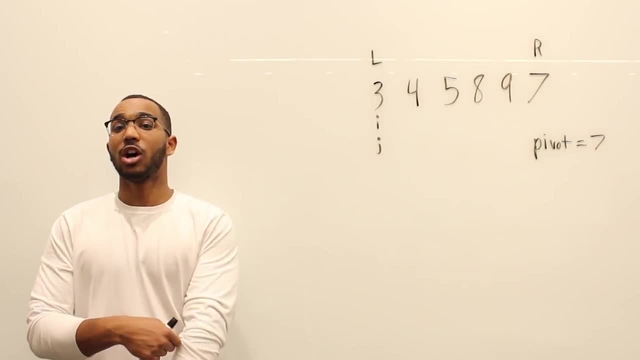 start here. it can start one behind. depends on your indexing. All I's job is is to remember the last place where we put the item less than a pivot. It's just keeping the tail of the linked list of items less than the pivot, if that makes sense. 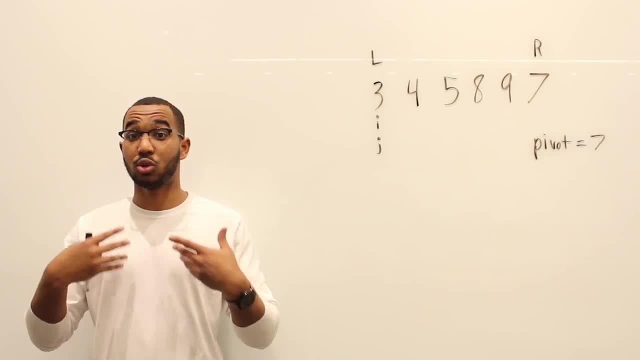 It's just keeping track of the tail, because that's where the pivot needs to be swapped into right. So what we need to do here is we need to look at this and we need to scan and we need to do swappings. So what we need to do is is: three less than the pivot, seven Yes. So what we're? 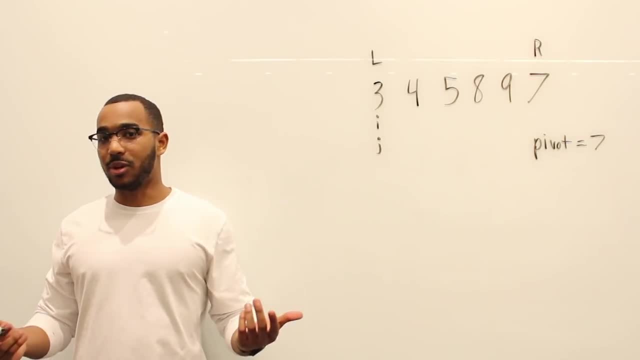 going to do is we swap I and J. We have nothing to do here because I sits on J. So if you're going to advance, J is four less than or equal to seven, Yes, So swap I and swap J, And what we need to do is 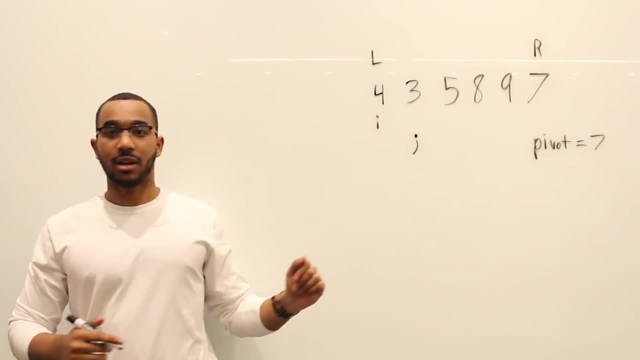 we advance I because we just did a swap at J and we need to advance J because J is our scanning guy. We don't need to sit here. We already looked at the element there. So now the last position of a swap is where I sits. The next item to investigate is where J sits. J is the investigator. 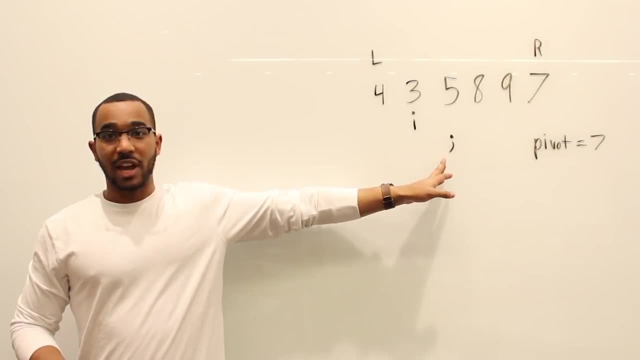 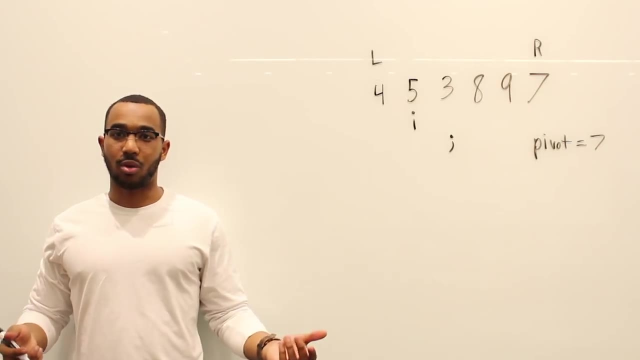 I is keeping memory Simple. So J five, is it less than or equal to seven? Yes, So swap five and three. And where was the last swap we just did? It's right here, where J sits, Move I And again. 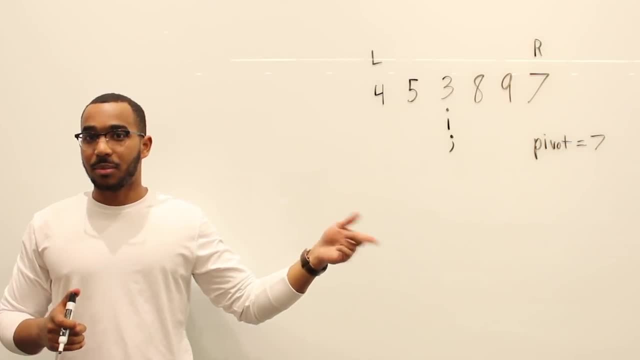 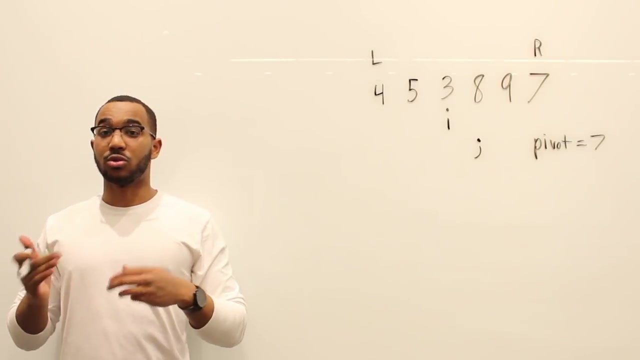 it's not dictated by J, We just increment I, because the next position we place in is the next position after I right. It just happens that that's where J is sitting. So what we do is: J is eight less than or equal to seven. No, it's not Advance. J Is nine less than or equal to seven. 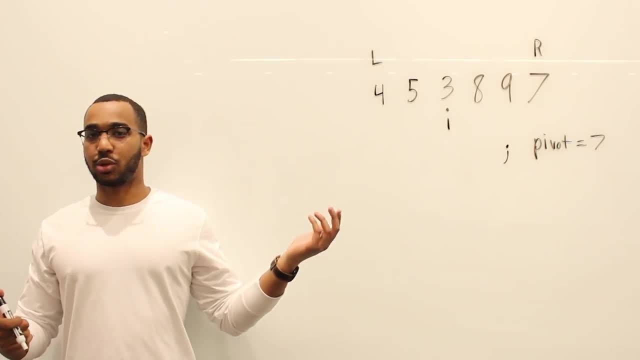 No Advance J J exhausts itself because it can't touch the right boundary, And I really, really, really want you to see this again. And this time we chose a better pivot, because this is what the partitioning looks like, or the- I keep saying partitioning. This is what the split looks like. 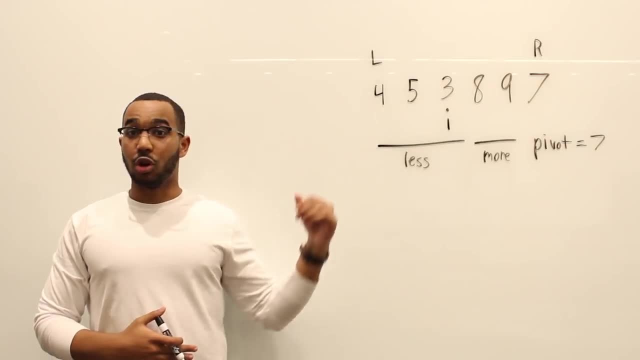 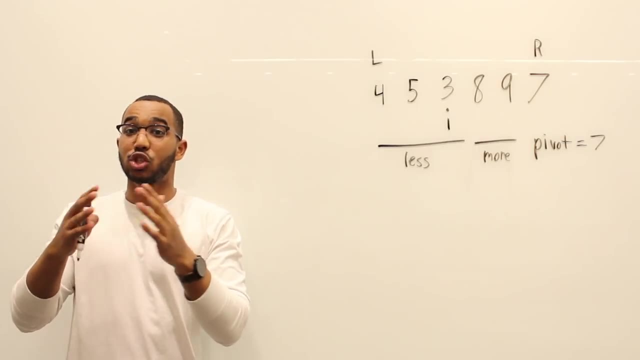 So all the items less than the pivot, those are sitting right there. All the items greater than the pivot are over here. So what we're going to do is we're going to go ahead and we're going to do. you see, do you see what I mean? J's job is to scan and say: Hey, I found an item less than. 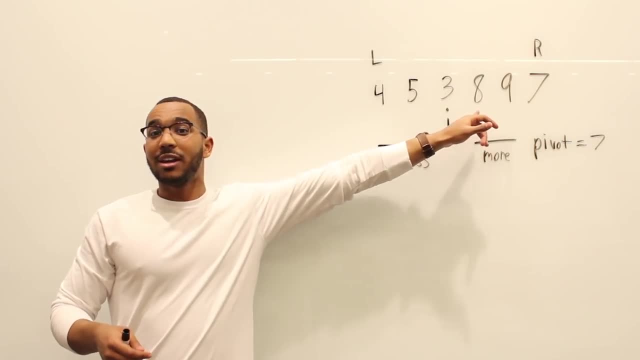 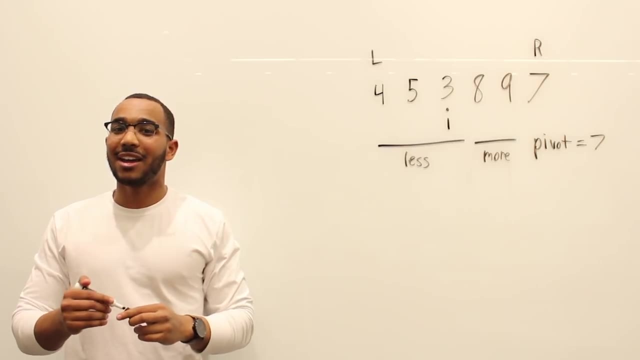 the pivot. Let me throw it back to you. I, we, we throw items back towards I so that we collect this section of items less than the pivot. And what is I sitting on? And this is very important And this is why I wanted you to see this: I is sitting on the tail of the items less than the 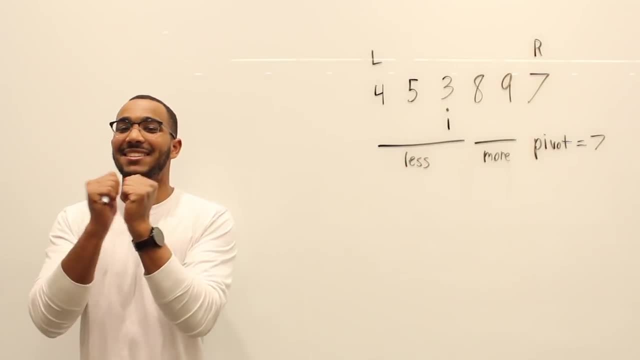 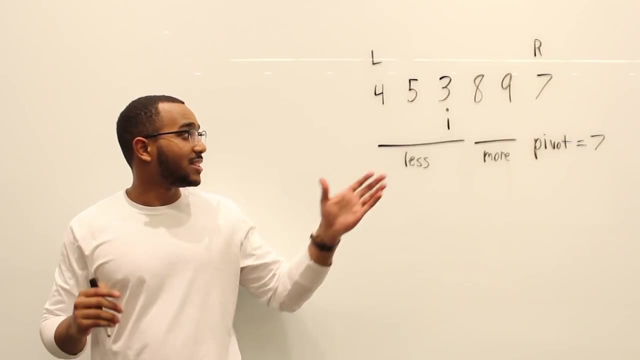 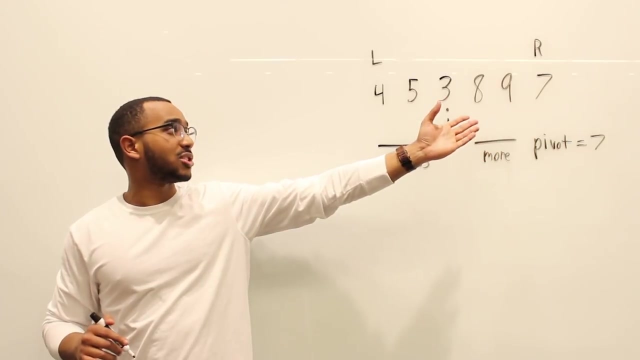 pivot. So where does the pivot go? It gets sandwiched between the pivot and the pivot, And so what I need to do is I need to swap the pivot into the section after it- And I probably messed this up in the other example- but you need to swap the pivot value, which is seven, with I. 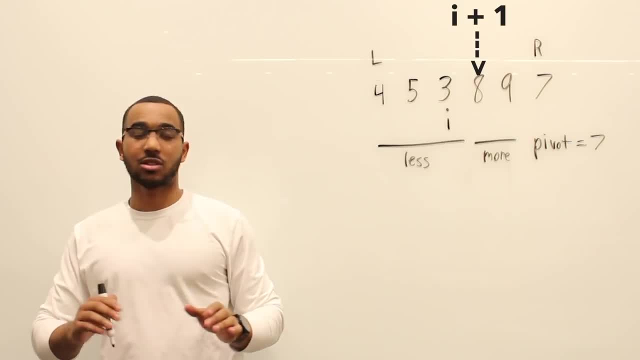 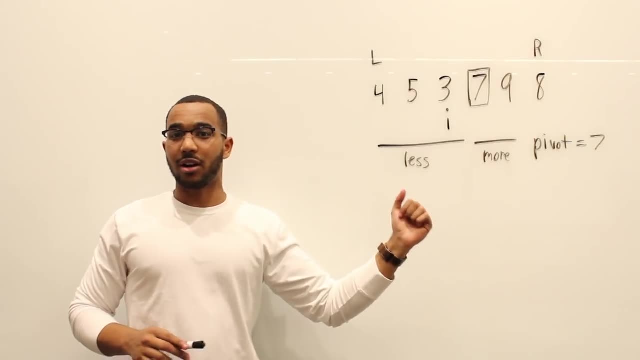 plus one, which is this value, sitting right here. So it looks like this. So, as you can see, throughout all of this, all these items are less than the pivot. All of these items are greater. And do you see how, if we call quick sort on this half and then this half, we're going to see that the 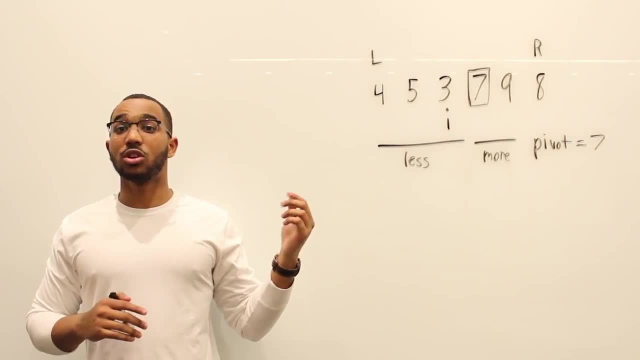 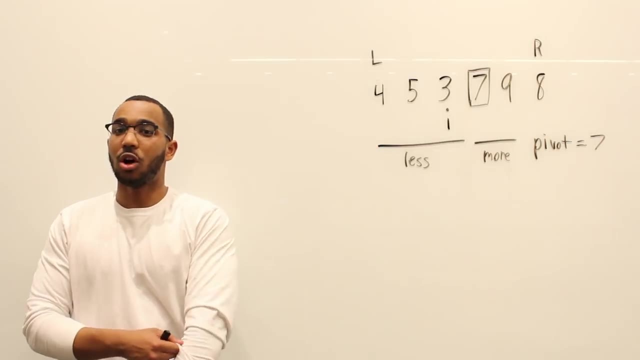 pivot is less than the pivot, and then this half. we're going to have relatively even halves. So this was a good pivot We just chose. So what we need to see is this is the intuition behind quicksort. It's all about cutting the space into items. less than an item, more than an item. 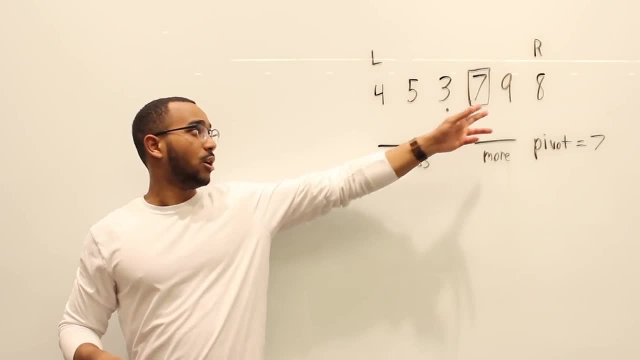 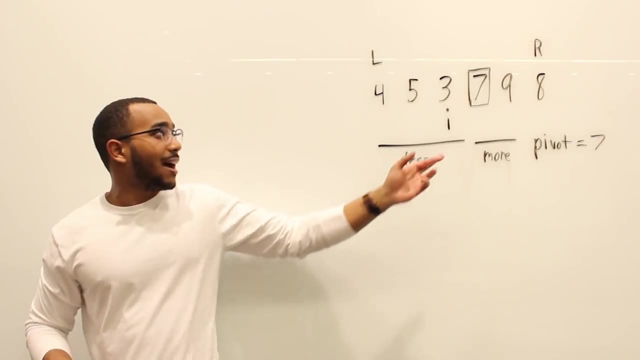 And this is how it happens recursively. We'll call quicksort here, We'll call quicksort there, and then it's going to do its thing and then return the index and then split downwards more And notice how we would return that index. We would split here, split there. 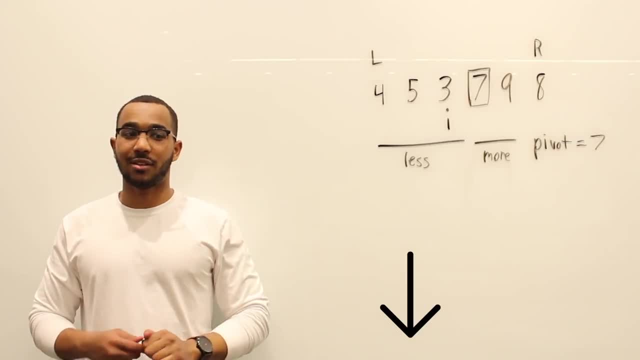 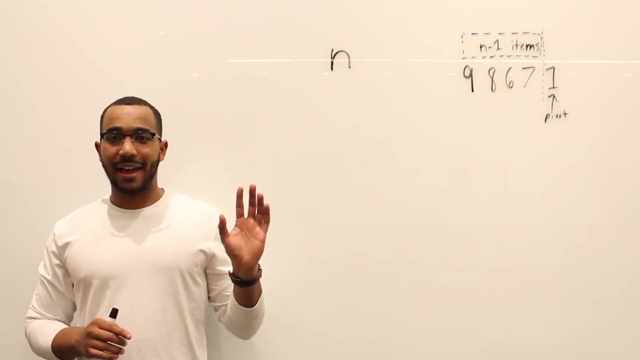 So again, code in the description to get a deeper understanding of that. So now let's look at the worst and the best case- recursion trees for this- and see why we get the runtimes that we eventually get. So let's look at that now. Okay. So now we're going to look at the worst case where we 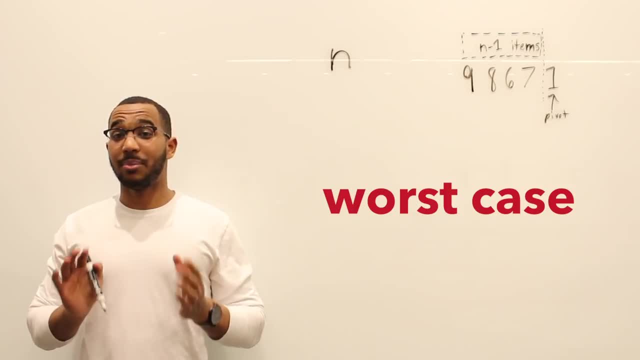 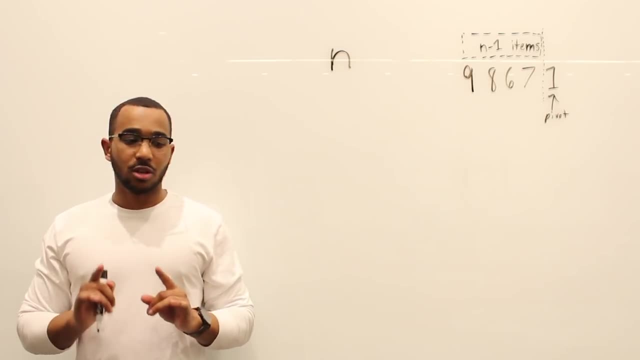 continuously, continuously, continuously choose bad pivots. A bad pivot is the largest item or the smallest item in the partitioning space. So what will happen is, let's let's look at a tree of this and see the size of the input as we make. 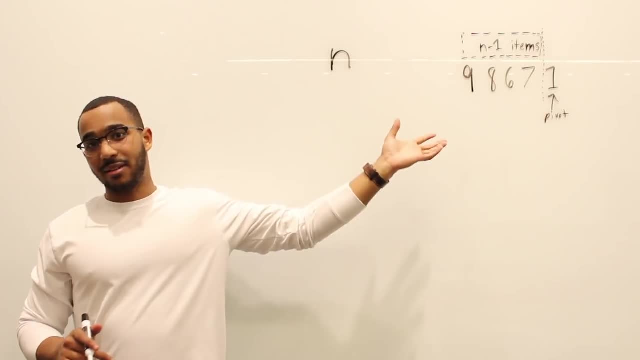 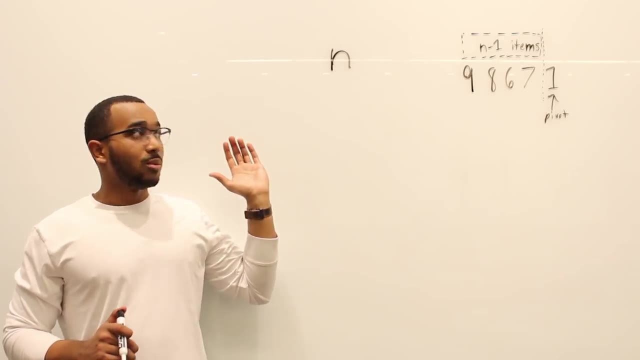 more calls to quicksort. So size of n. if I choose a bad pivot, like in this top level, uh call, if I choose one as the pivot, I'm going to do my n minus one comparisons and my pivot value. 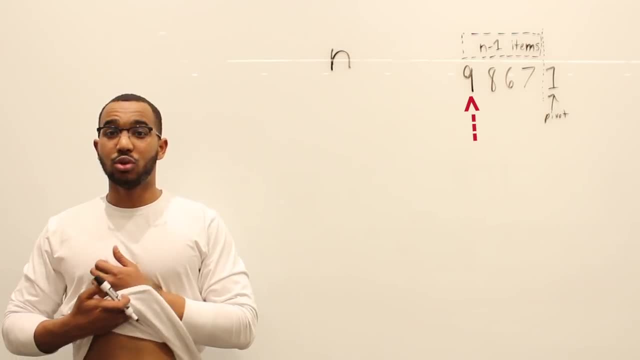 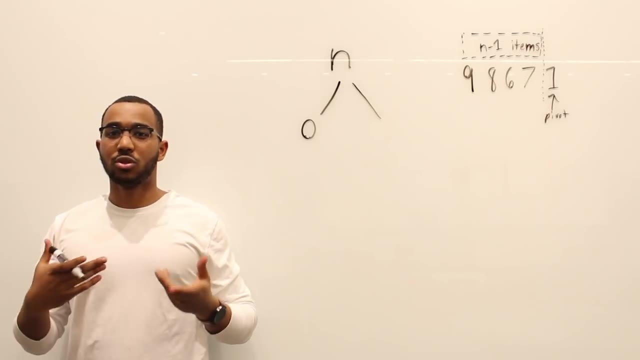 I'm going to find out is that index zero. I'm going to split to the left and the right. I'm going to split to the left with a base case of no items, And then I'm going to split to the left with n minus one items, And then I'm going to split to the right with n minus one items, And again. 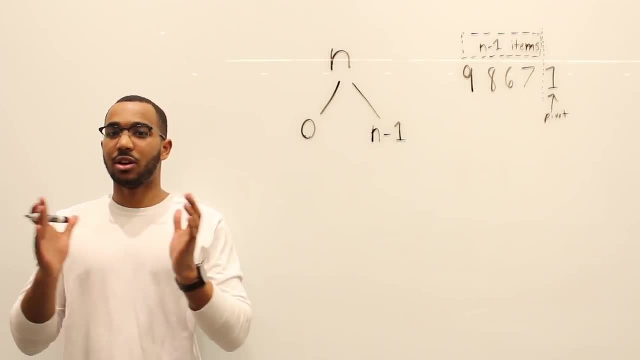 we're looking at the amount of items um considered within each call. So what we do is, if we pick another bad pivot, we're going to split to the left with zero items, And then we're going to split to the right with n minus two items again. 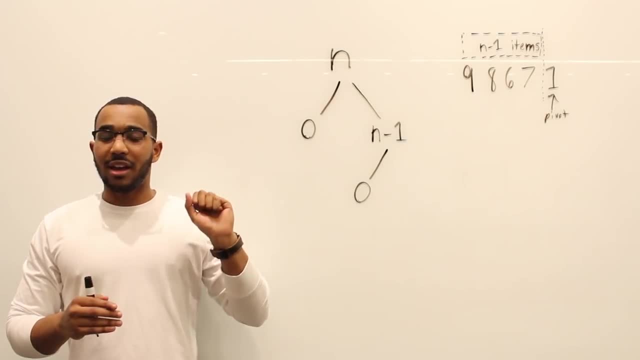 because we're going to have one less item, If that makes sense, each time we place an item we're going to have one less item. So the next call we'll just have one less item, because this tree is very skewed, because we're choosing bad pivots. 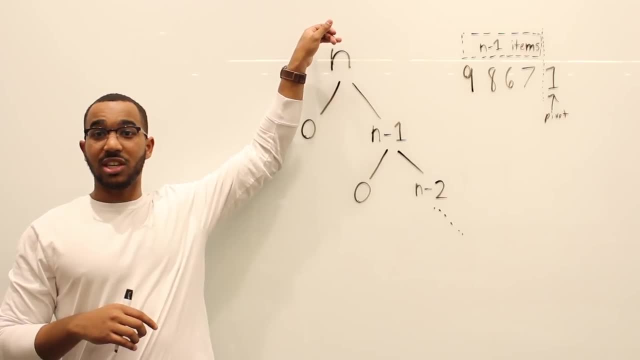 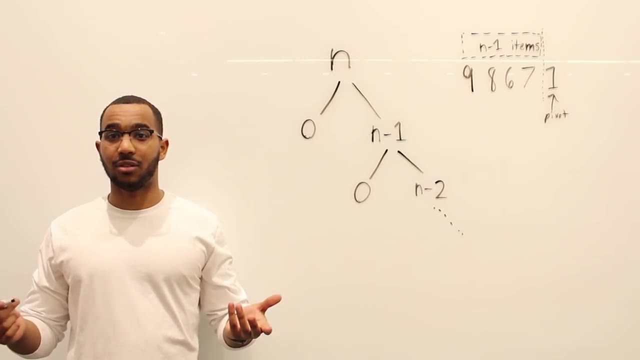 So that's going to keep going And what we're going to do is we're going to continuously split our input downwards, And what's going to happen is we're going to be doing how much work at each level, So at the top level, and items we will do. 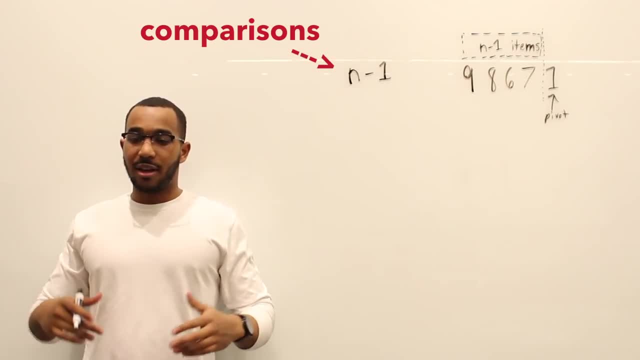 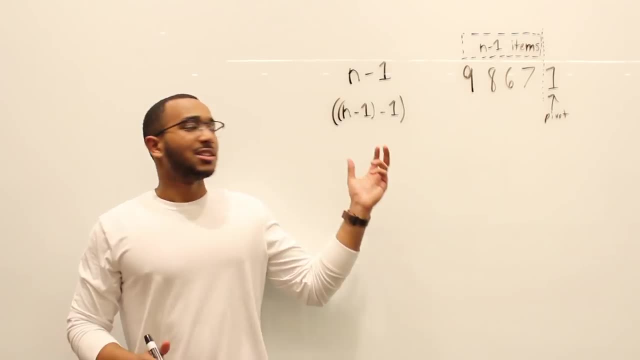 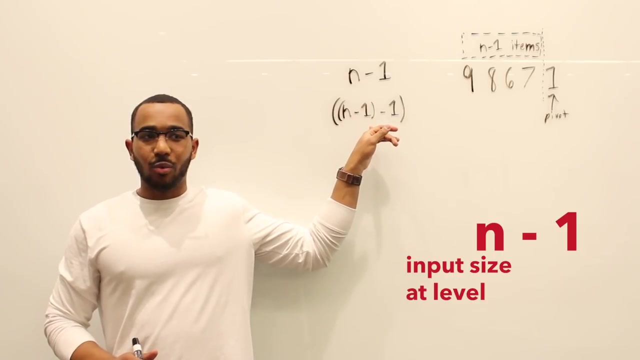 n minus one work. top level: We do n minus one work. the next level, down, We're going to be doing n minus one minus one work. Stay with me. Does that make sense? So we, the input size at the next level is n minus one. But then what is the work that we do? 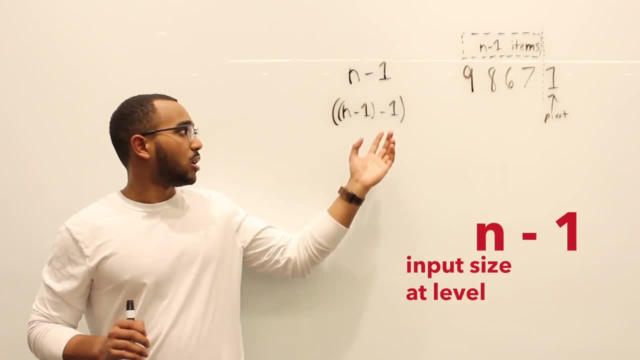 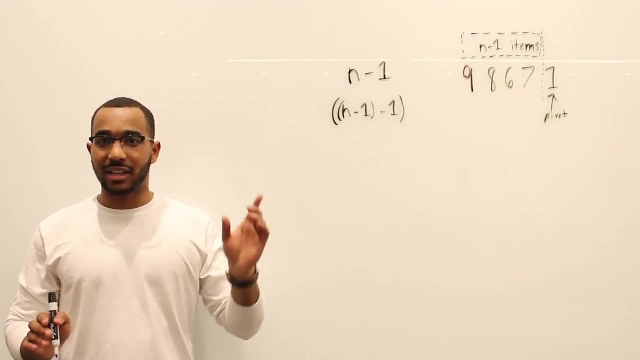 in that call, The only call in that level that yields work. we're going to do n minus one. So we plug in the size of the input And again we've done analyzing recurrent recurrence relations and re recursion trees. So this is no different. We see that this is 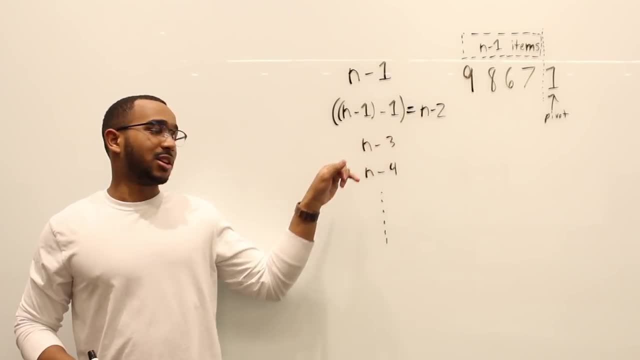 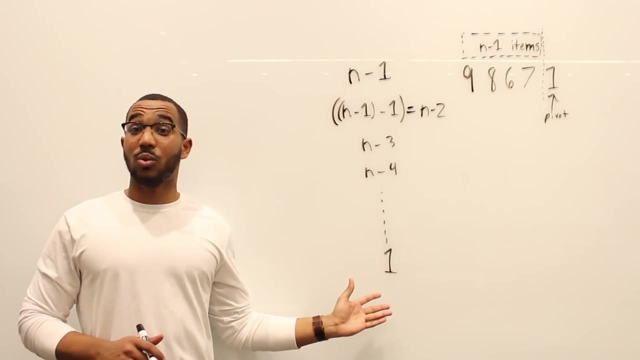 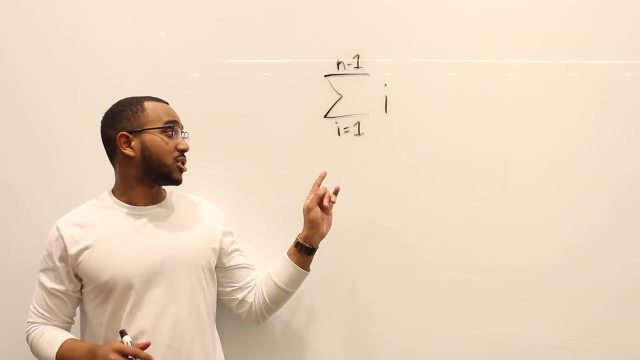 just n minus two. So we're going to do n minus two work and minus three and minus four and so on, And what you see here is we go from n minus one until we get down to one item, But we know how to do summations. What is this actually saying? That is what this is actually. 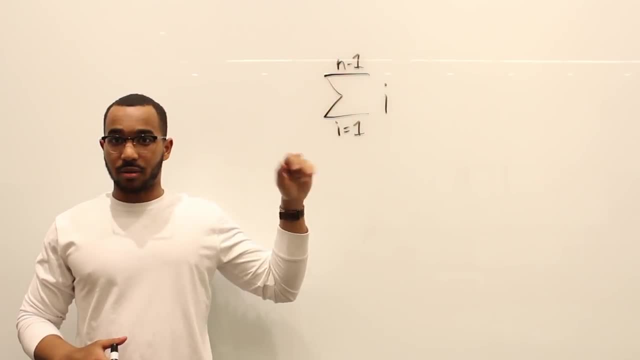 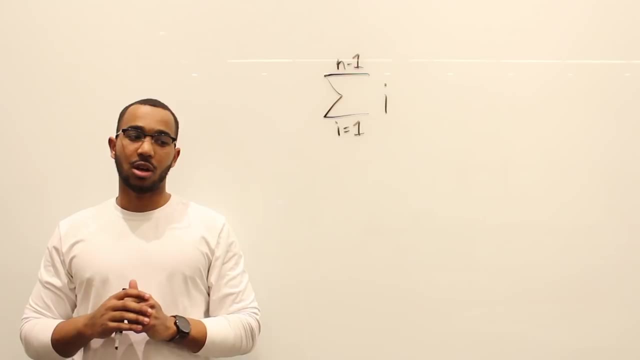 saying The summation from one to n minus one sum the work from one to n minus one. That is going to sum the work in that whole recursion tree we just saw. So what is this equal? We already know that we can use a Gaussian sum or we can use Gauss's trick to solve this. 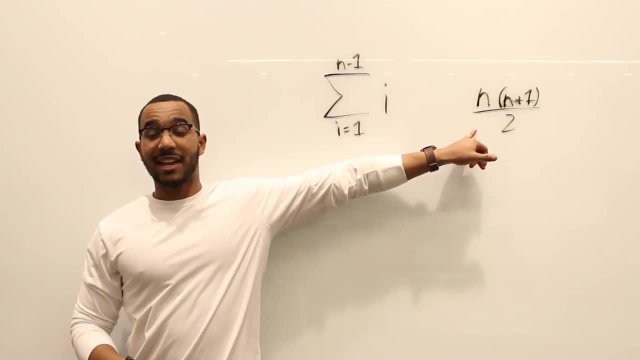 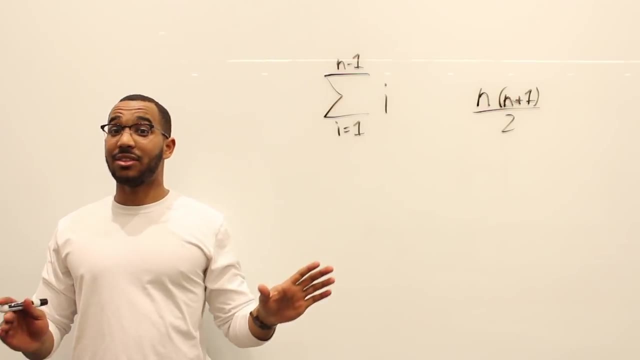 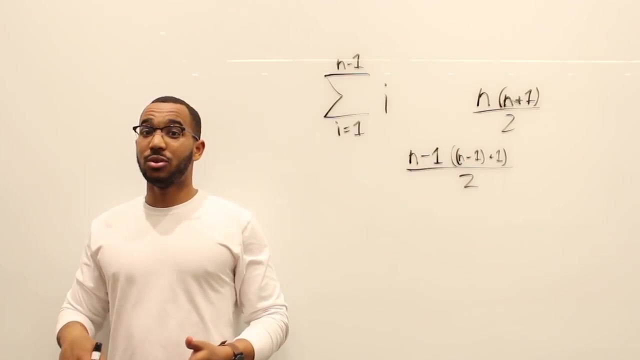 Where our value to plug into this. that's Gauss's trick. We plug n minus one our upper bound, our top bound, into n right there, And we get this. We get n minus one times this, n minus one plus one over two. What does that simplify to? What that simplifies to is n minus one times n over two. 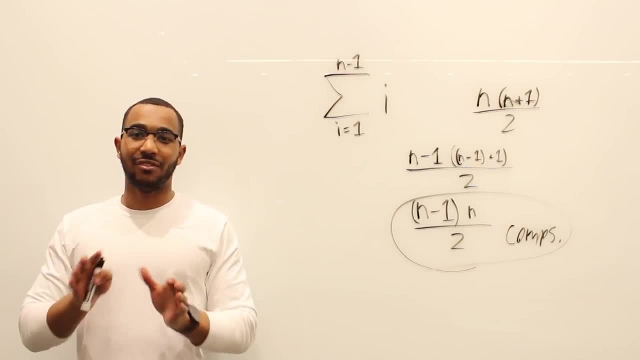 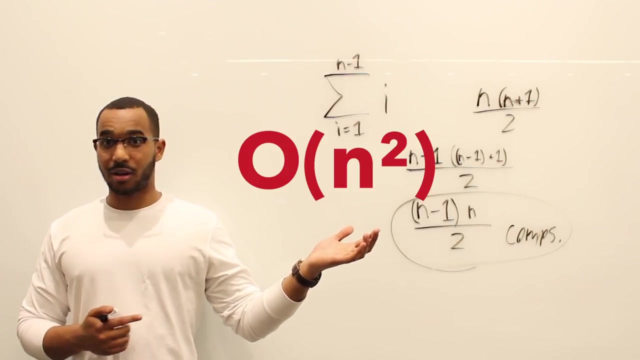 Comparisons. at worst, If we choose a bad pivot, every call we can upper bound the worst amount we do to this amount. So what does that? let us make our big O upper bound if we're dropping our constants and everything That is big O of n squared. So that is why quicksort runs in big O. 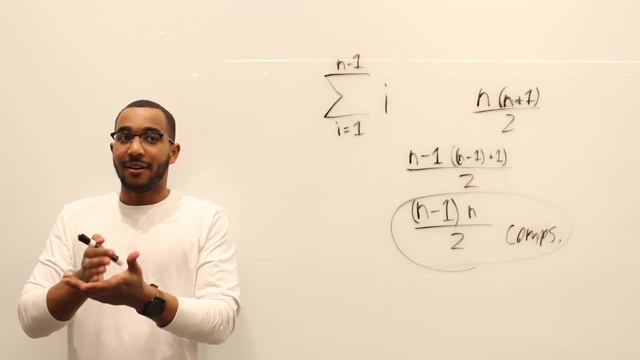 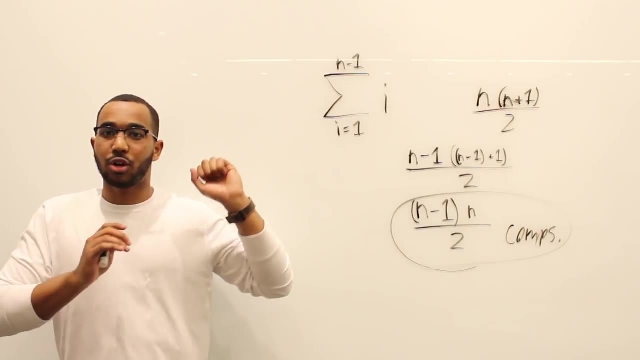 of n squared. In the worst case, we're going to be chopping in half very unevenly, as unevenly as possible. Every time we're going to reduce the input size by one and we're going to make our recursion tree really, really deep, And that's bad. 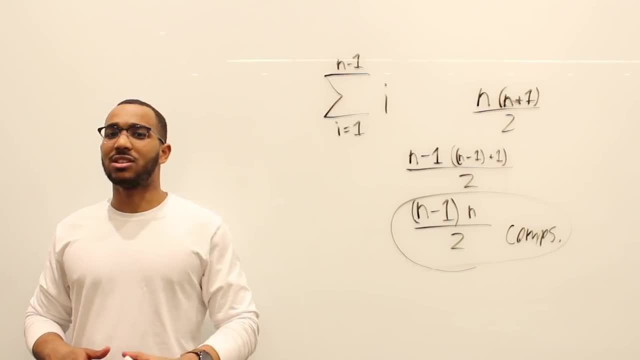 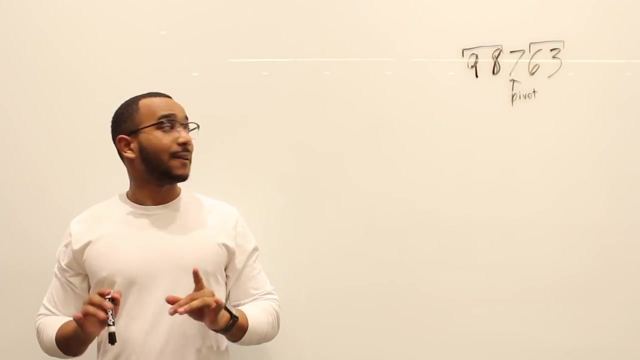 We see the worst case. So now let's look at the best case, the best way quicksort can perform. And this is when we pick a pivot that is good, And we're going to look at what that means now. Okay, So if we pick a good pivot, what is a good pivot? A good pivot is the median. 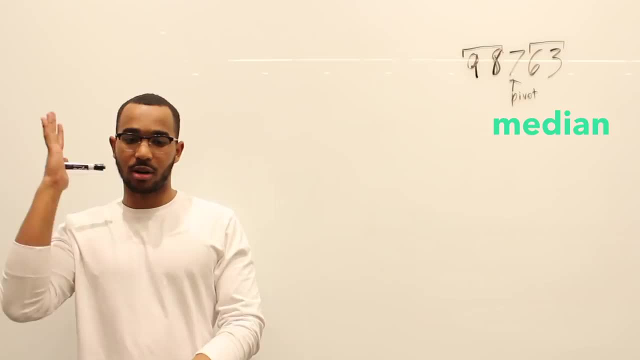 of the partitioning space, the median of the space that we are looking at. So what is the median of that set of data? If we put it in order, look to the middle, it'd be seven. And again, do you see how I chose this pivot? It's not the last item. 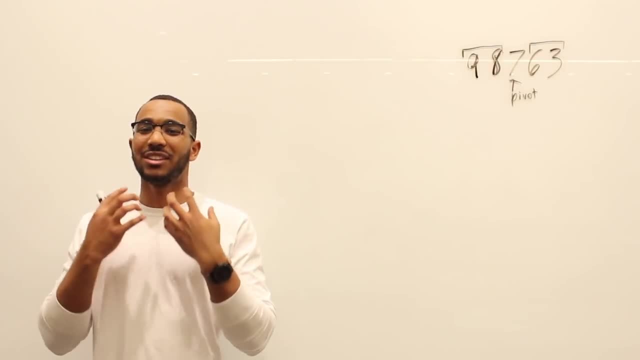 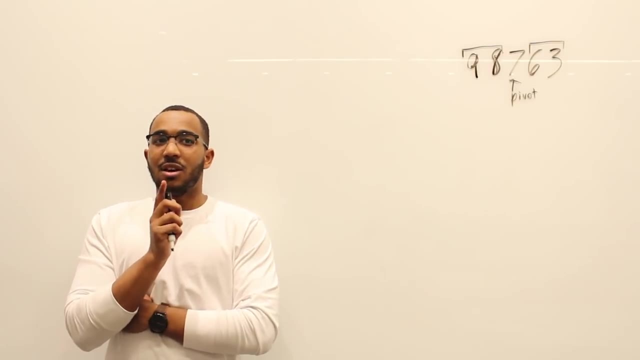 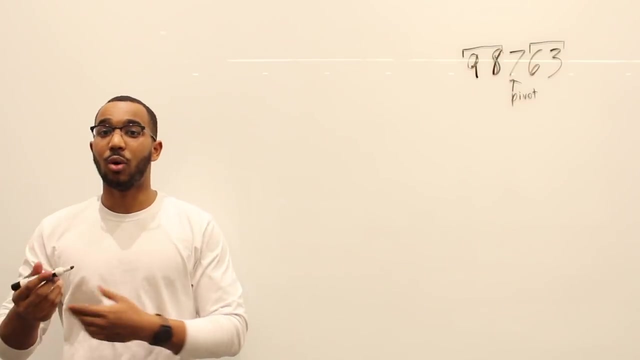 We can choose any guy as the pivot, It does not matter. That is actually the fundamental question. Choosing good pivots makes this algorithm more optimal. So what we need to see is: if we choose a perfect pivot every time, choose the median every time, what will the runtime look like? 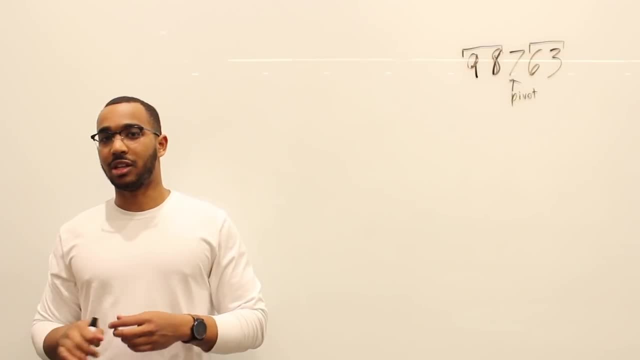 And it's going to look like an algorithm we already know, but you'll see in a little. So let's start with our input size. So size n. And now if we go left, what will the size of the input be? If we go to the left? 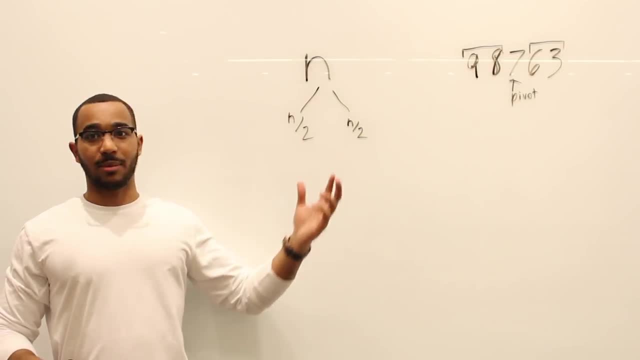 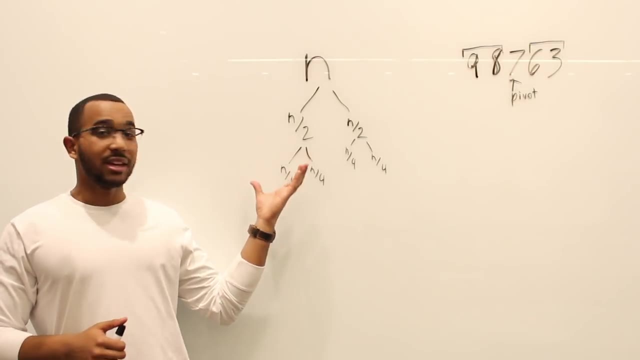 we split the input roughly in half. If we go to the right, we split the input in half And what we need to do is do another splitting. So if we split the input in half again, we get n over four as a layer, And what we need to do is we need to see how much work is done in. 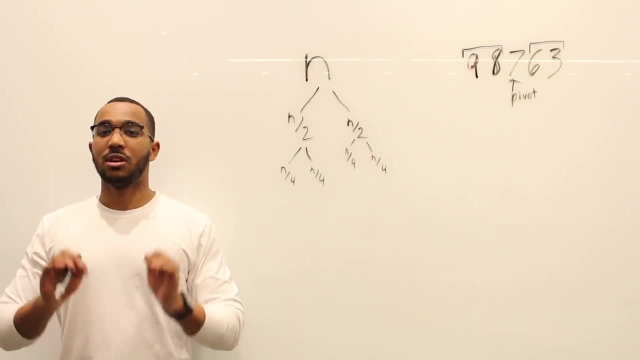 every layer. Again, we're picking perfect pivots, median pivots, and it's allowing us to split this space perfectly. So if we go to the left, what will the size of the input be? If we go to the right, we split the input in half And what we need to do is set up a pivots in half. So if we go, to the left. what will the size of the input be If we split the input in half? again, we get n over four as a layer. Again, we get n over one as a layer, And what we need to do is split this. 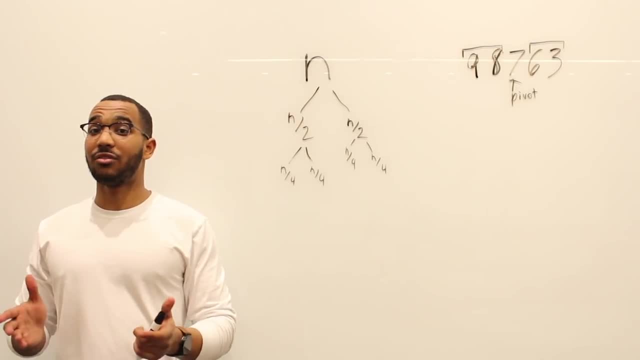 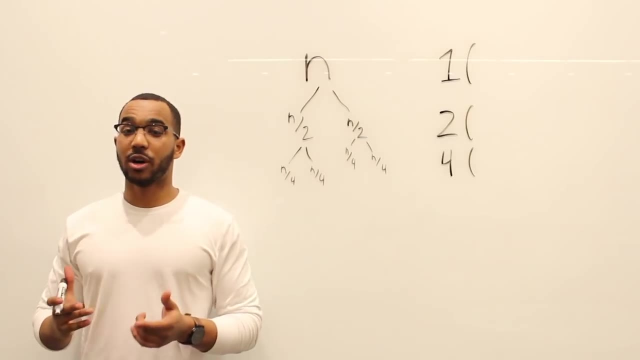 space perfectly. So what we need to look at is the work per level. Okay, So one sub problem, two sub problems, four sub problems. How much work is done in each sub problem? So, at the top level, n minus one. 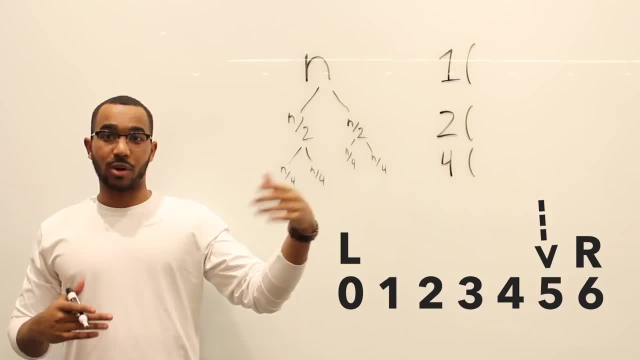 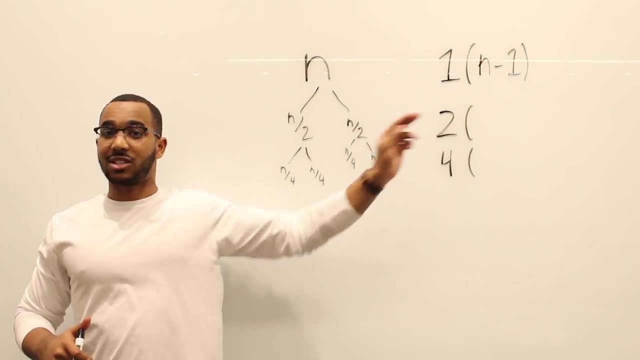 remember, we're going from the left boundary to r minus one, which is n minus one. comparisons: Next, we're not doing n minus one. in the next level, We're going to be doing n over two minus one, because this is the end of the equation. And this is the end of the equation, So we're going to. 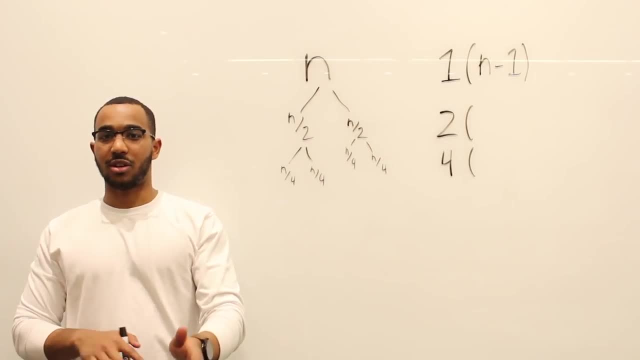 this is the input size to the partition function And it'll tell us how many comparisons we do right. It depends on the size of the input in the sub call. So it becomes N over two minus one and then the next level, N over four minus one. 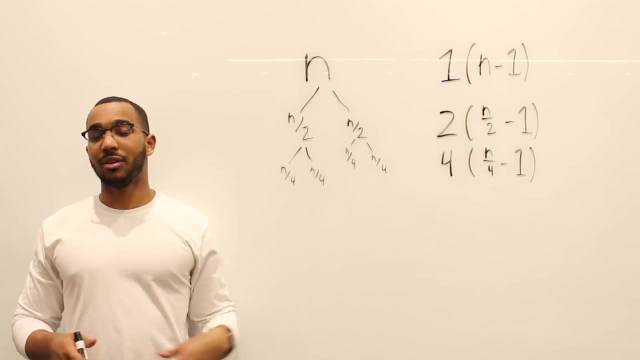 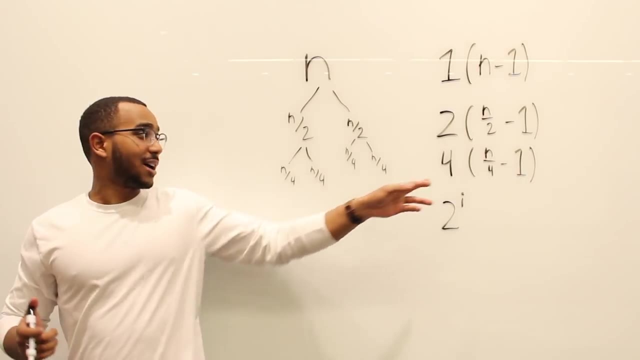 And then now we can see a pattern. We generalize the number of sub problems, which is two to the I, two to the number, to the level we're on. And then what we also do is we generalize this guy. It becomes N over two to the I, minus one. 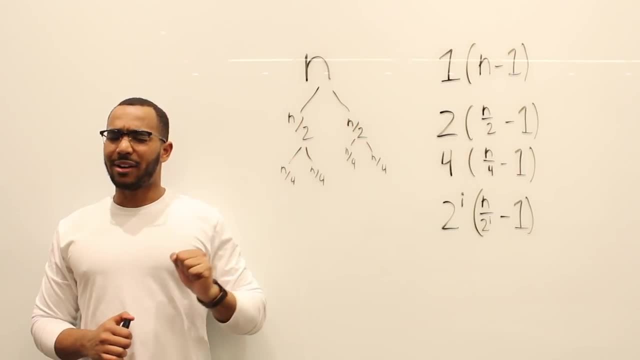 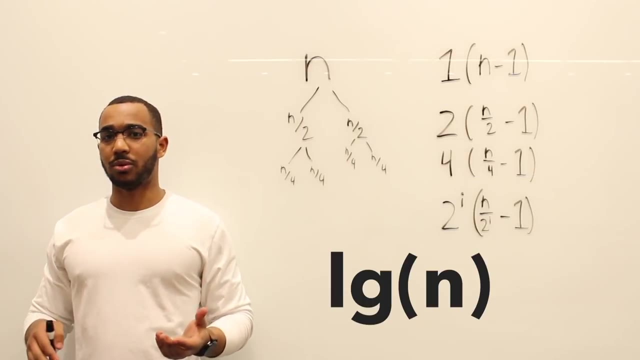 And how many levels will we have? Well, we're forking, we're having- And I've done videos on logarithms before and we know what having means. It means log base two. It means we're cutting in half. And how do we understand how many times we can cut in half? 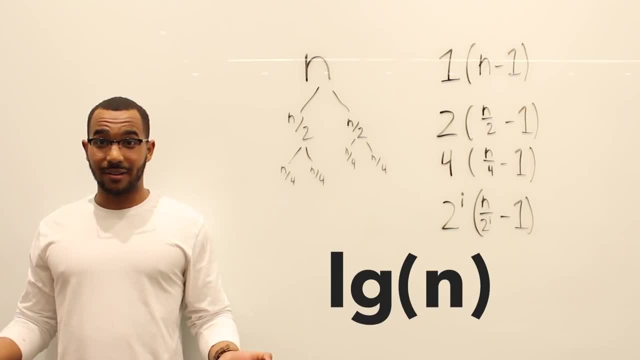 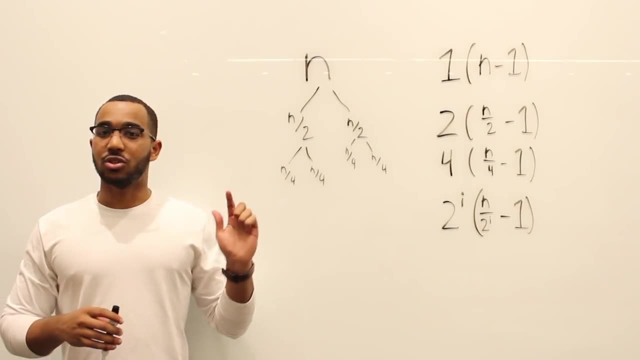 We use log base two, a logarithm. So log of N, log base two of N, will tell us how many levels there are in the tree. So what we need to do is we need to take the sum of the work at every level. 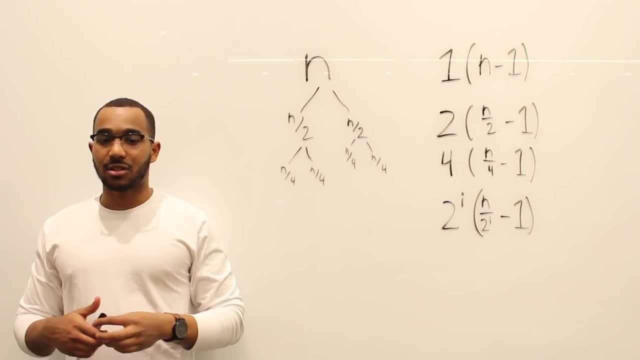 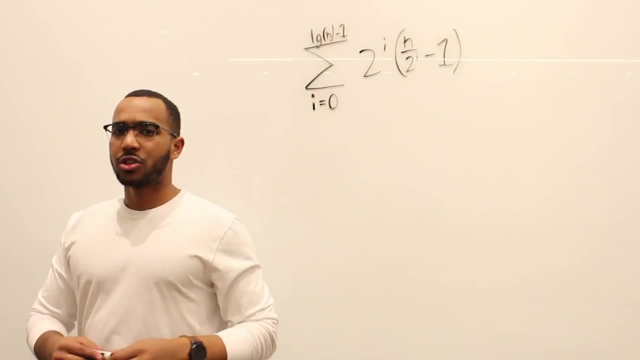 we generalized it and that's going to give us the exact upper bound on the worst work that the best case can do. So let's do that right now. So how many comparisons are done at the base level, the leaf level, I mean, if we really think about it? 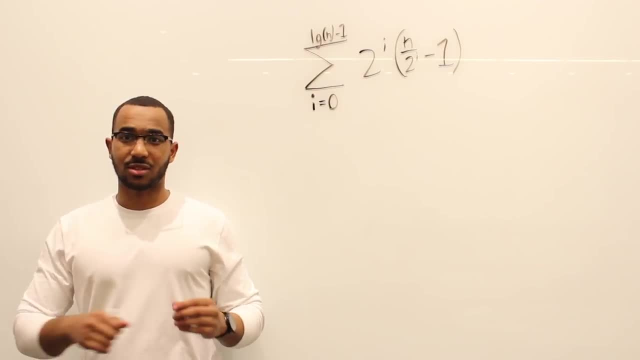 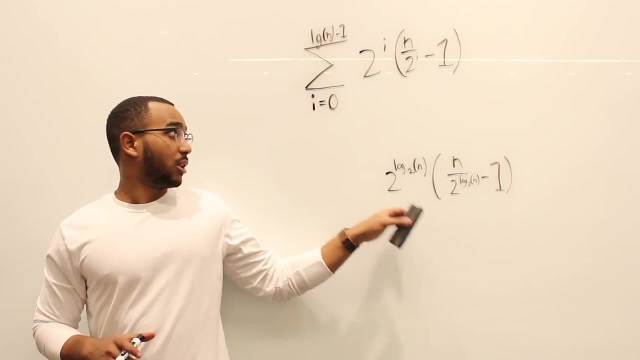 what we're going to be doing is: we're going to be doing this, We're gonna be doing that, And I just wanna touch on this real quick. So this is the work we're going to be doing at the leaf level. We're just taking the generalization. 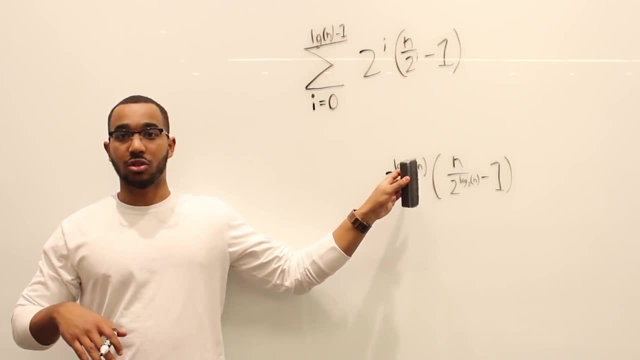 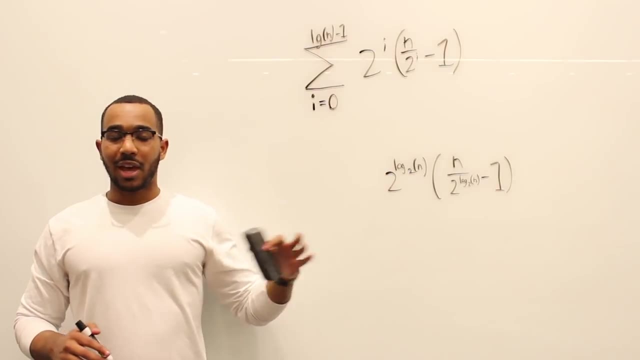 and plugging the level number, the last level, which is log of N, the log of N level, the last level. We're going to plug that in And what we're going to see is if we add two to the power of a logarithm. 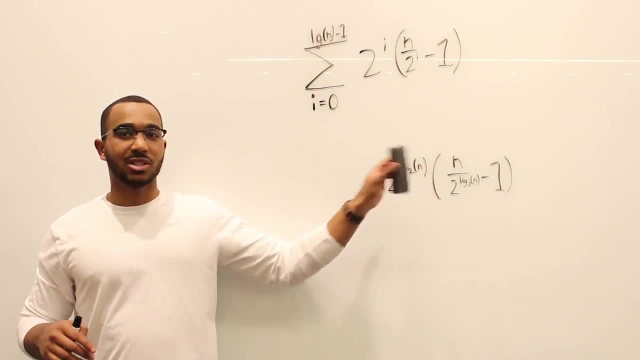 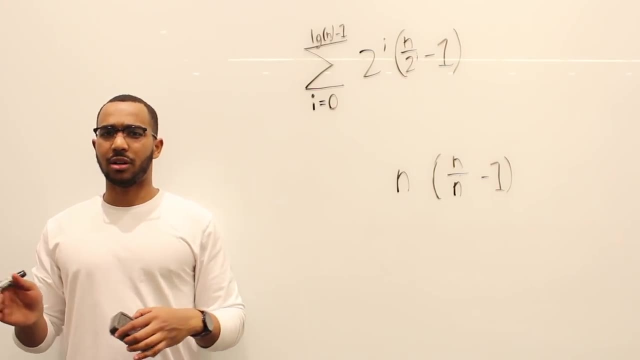 with the same base value as that number, it just becomes the value inside the parentheses of the logarithm, which is N. Same thing here, And then N over N is one, One minus one is zero, And then N sub-problems times zero work done. 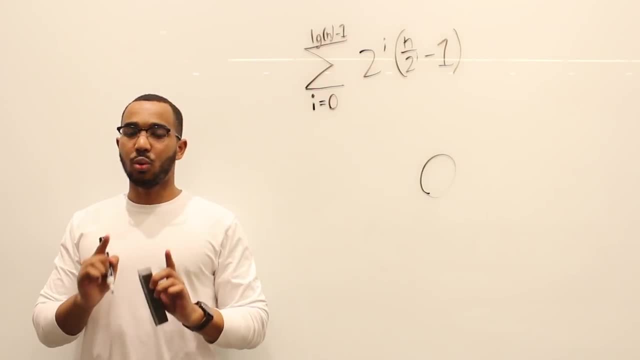 per sub-problem is zero. So that is the work done at the log N level, the final level, And do you see how my summation stops and doesn't even sum the last level? It wouldn't matter if we summed the last level. 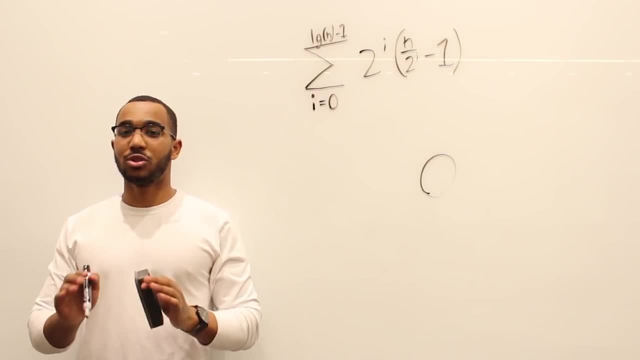 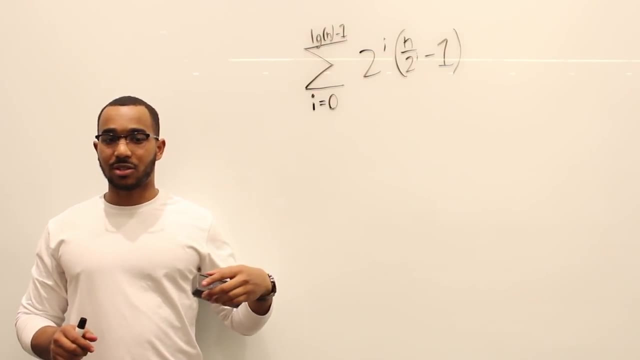 We would get zero work for it. It would not contribute to the sum. I wanted to address this because I might get a question about that tiny detail. So what we need to look at is how do we solve this, And actually I'm not going. 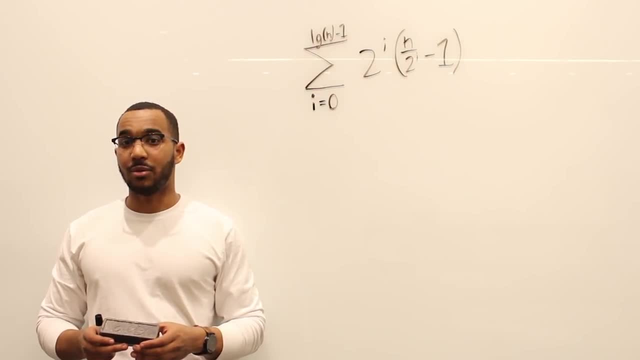 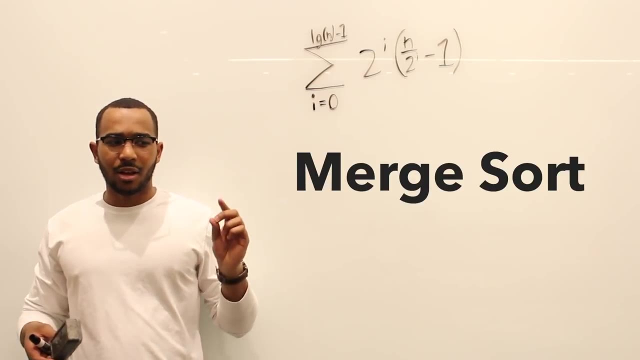 to solve this, because we know how to solve this already. We've seen this already, We've done this, And we did that in an algorithm called merge sort, And we have a video on that, And this is what the final solution looks like, right. 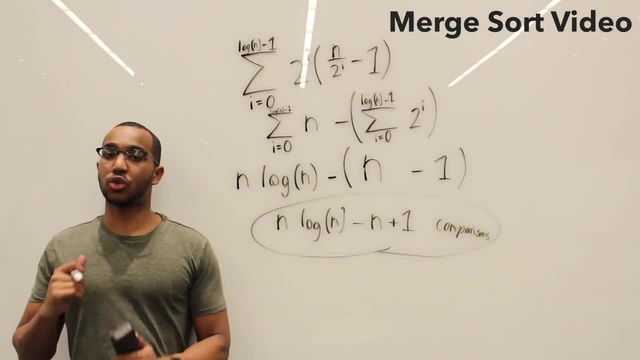 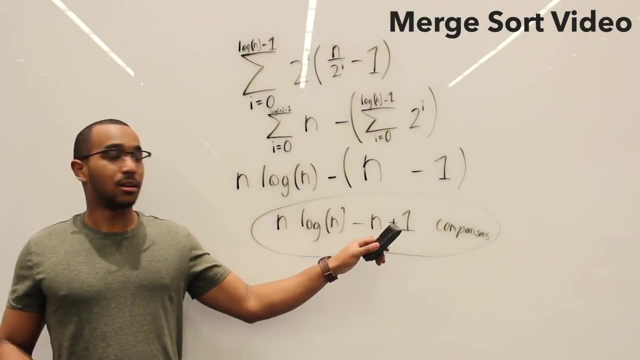 What do we find? So the amount of comparisons for merge sort, in the worst case, the upper bound we can provide is this exact amount: N log N minus N plus one comparisons. This is how much work we will do, total given an N. 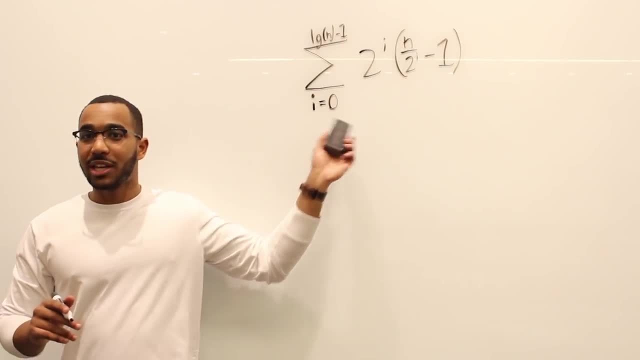 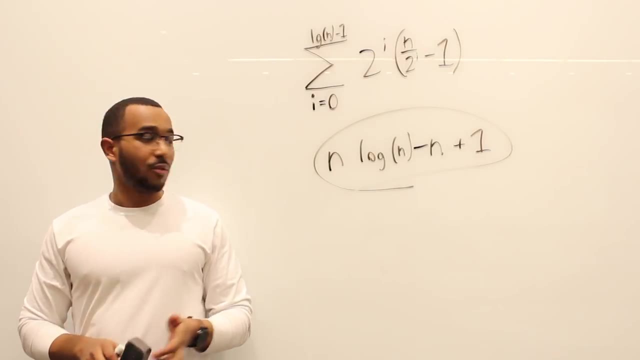 Okay, yeah, so that is the exact same thing we're doing here. So what's the final value? So these are the worst case comparisons for the best case of quicksort. It's the exact same thing. exact same thing because the recursion panned out to be the same. 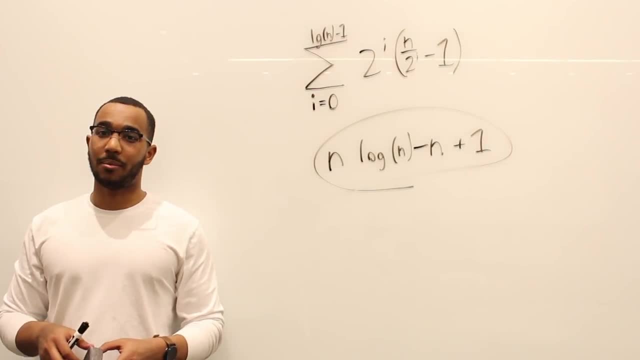 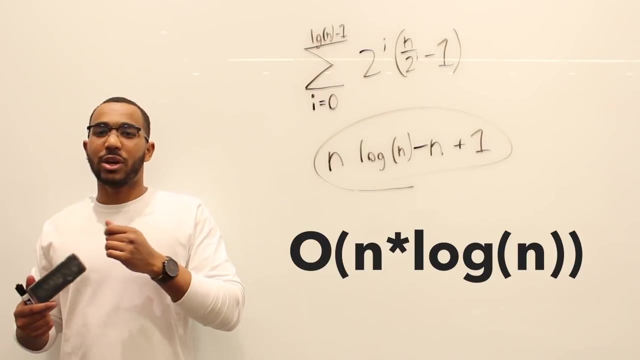 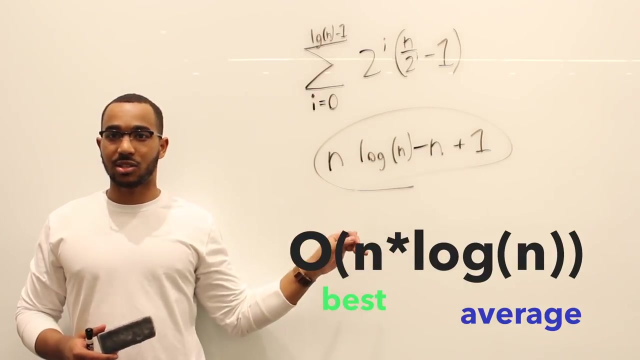 We're splitting and then we're doing a certain amount of work in each sub problem, So this can be bounded by big O of N log N. This is why quicksort, in the best and the average case, is big O of N log N, because it deduces exactly to this. 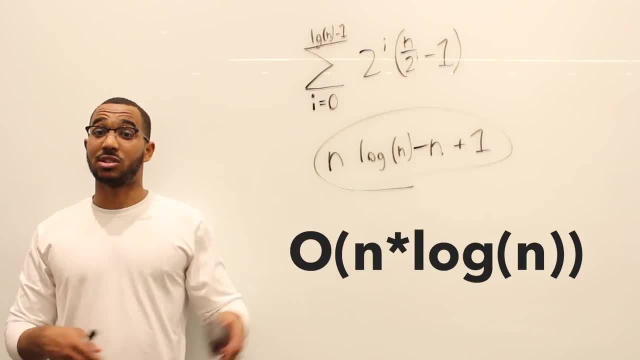 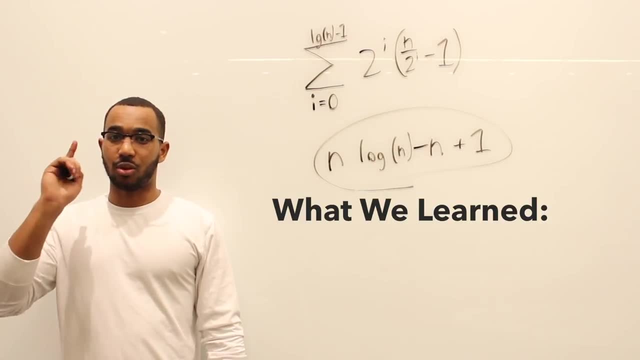 And then we bound to the highest order term, right there, because this is asymptotic And these guys don't matter. the minus N and one. So this is quicksort. We looked at the worst, We looked at the best case of quicksort. 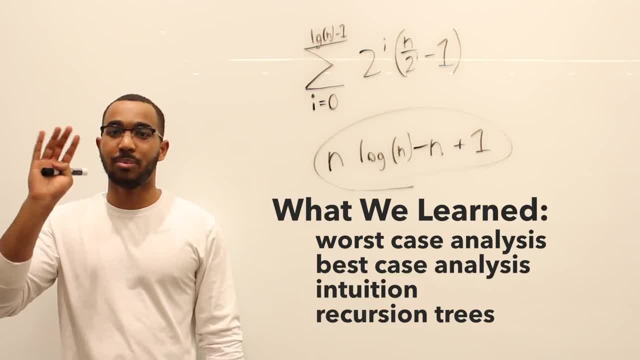 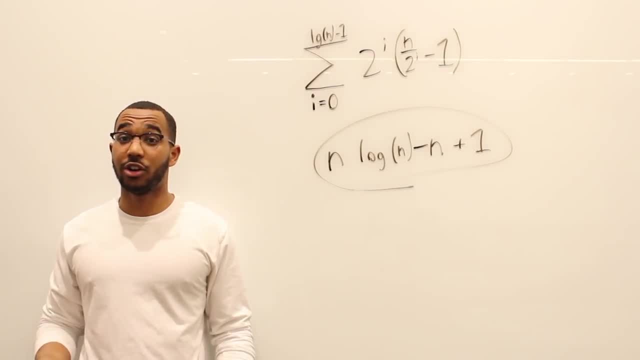 We looked at the intuition behind quicksort. We looked at the recursion behavior of quicksort. This is pretty exhaustively how quicksort works. You can investigate the code in the description. That will further your understanding. But this is the gist of it. 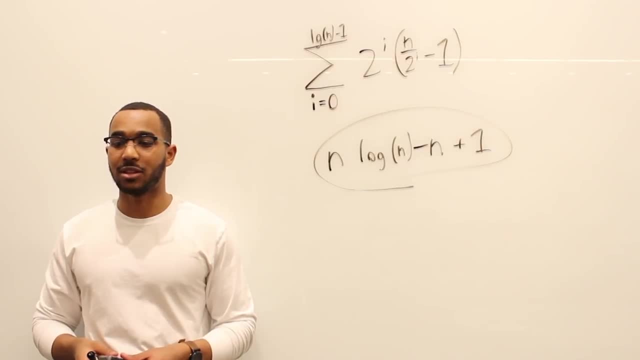 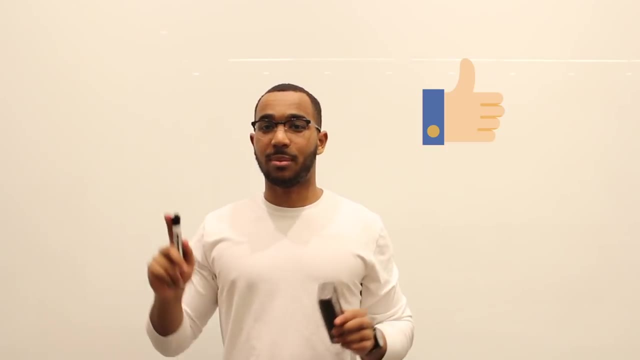 This is the deepest way I probably can explain this. Yeah, All right, so that is all for this video. If you like this video, hit the like button. Subscribe to the channel for more videos. I'm sorry I've been slowing down the video production. 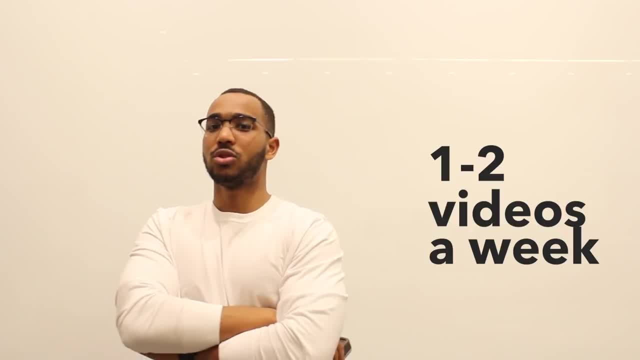 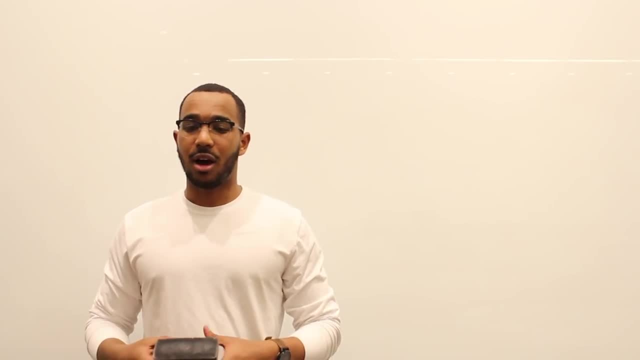 I'm going to probably be doing one video a week from now on, two videos at max, because I'm trying to work on a course with some friends that I want to have out in a few months. A lot of people have been asking me. 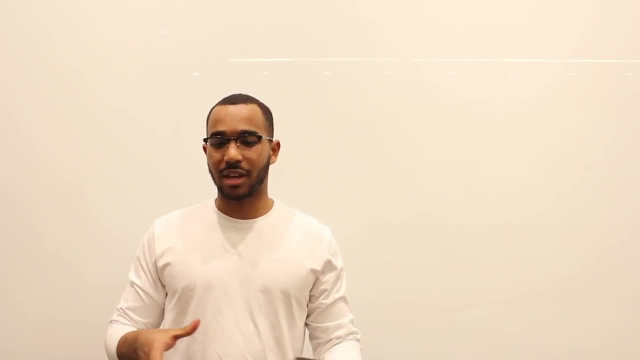 about, like coaching and courses, and I really don't like the coaching avenue because it's so expensive, because you can learn so much more. I'll be honest with you: You can learn so much more from doing LeetCode questions, from reading books like Elements of Programming Interviews. 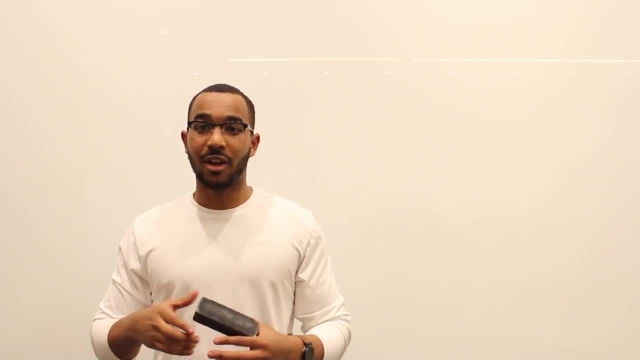 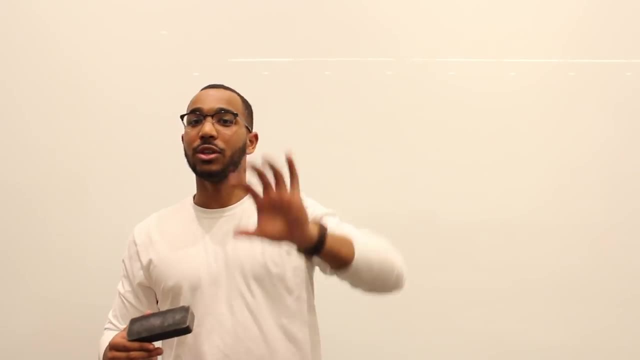 Cracking the Coding Interview. You can learn so much more from teaching yourself than doing some program or some expensive thing. that will give you the same value as struggling And going through the concepts yourself. So that's kind of my gist and I'm kind of saying that.